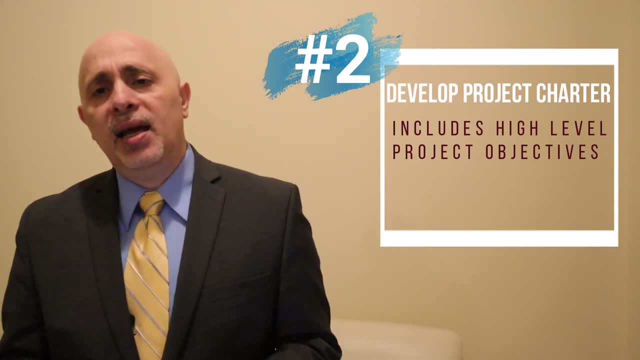 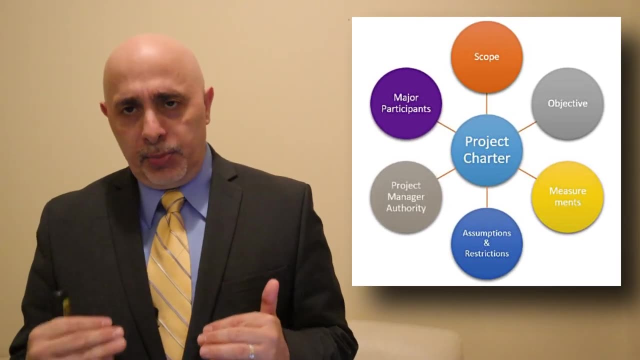 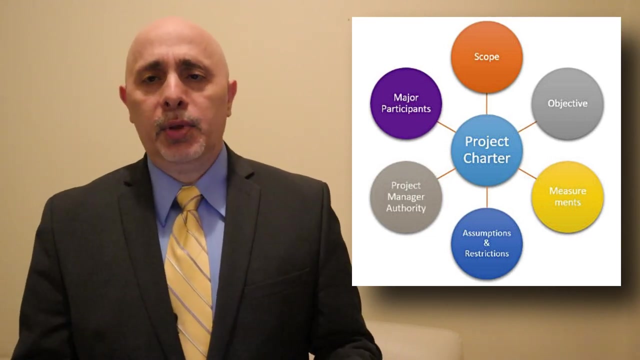 initiation document or a project brief, and it stands for a one page or two page document that includes all of the high level objectives of the project, Things such as: why are we running the project? like the justification, What is the end product, How much time are we going to have on it? 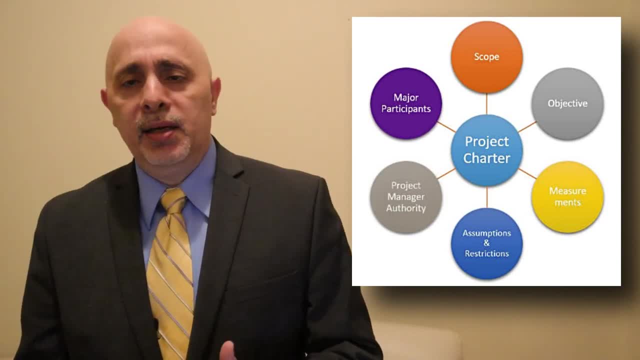 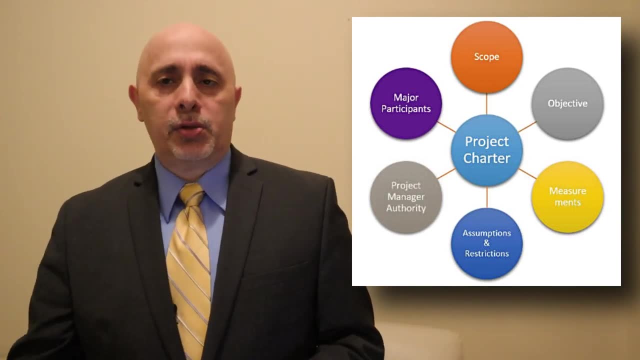 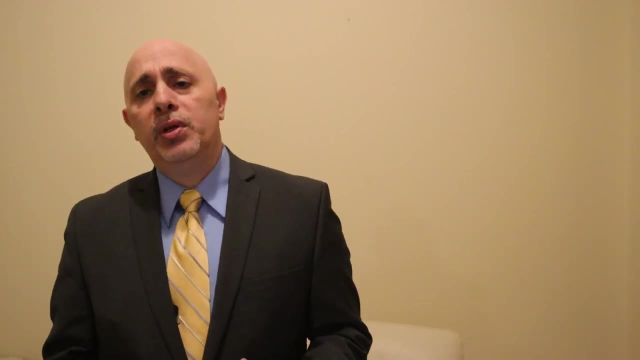 How much is the budget? Are there any key dependencies? Are we making any assumptions? Who are the key stakeholders in the organization that will support you on it? Are there some key milestones that they're looking to achieve? Now, once you have the charter prepared, what you want to do is you want to review this with 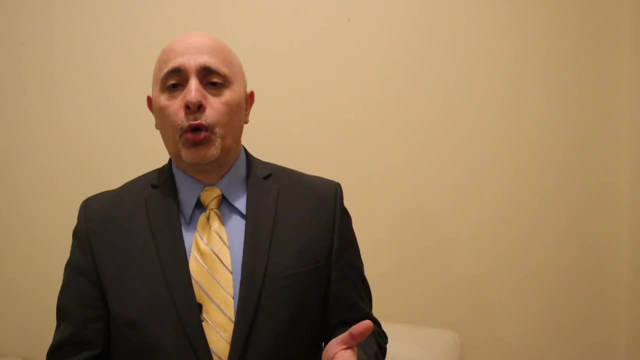 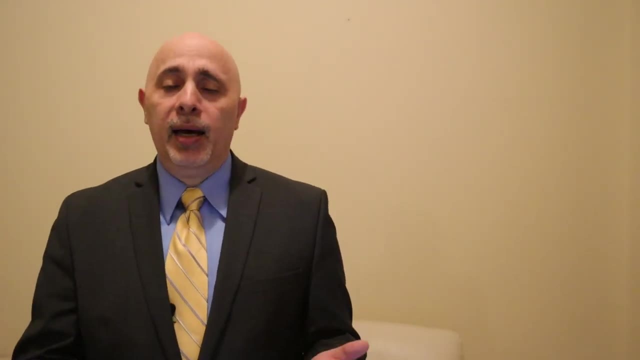 your sponsor, your boss, and have them go over it And if they're okay with it, let them sign it. Ask them to please sign that one document And if they can also send out an email to all of the top department managers and let them know that. 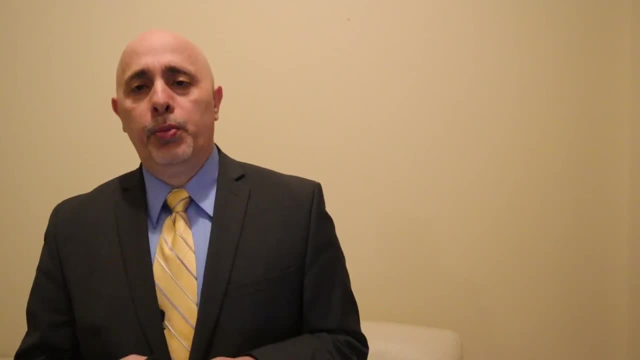 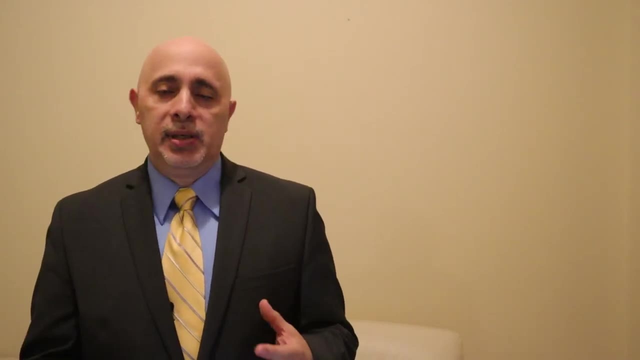 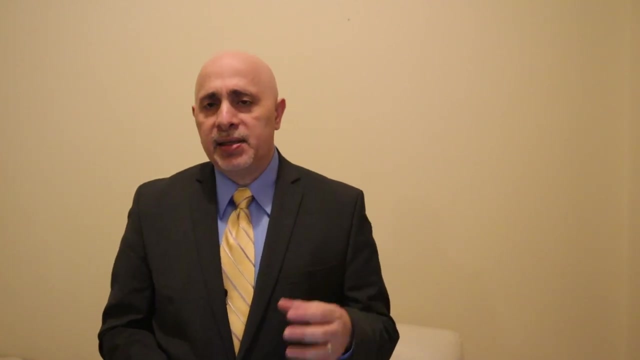 this project has been initiated and that you are going to be the project manager on that. That gives you credibility, for you to go around talking to different people and asking questions and asking to review some documents or existing processes. All right, So now you've been assigned. 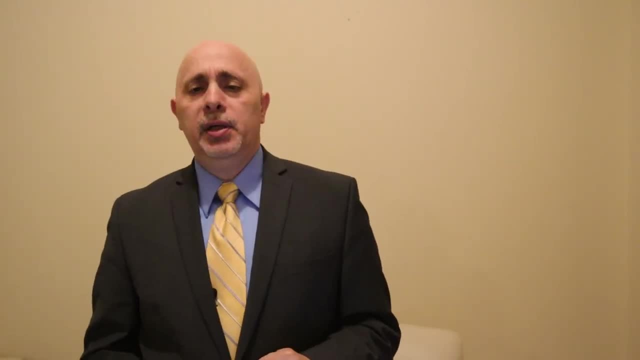 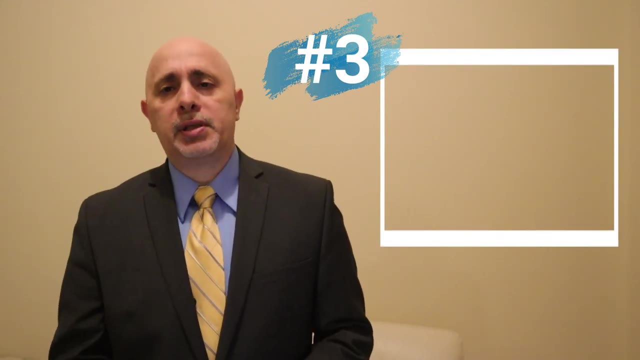 you've got all the details, you've developed a project charter and the next thing that you need to do is step number three. Step number three is to review the project, And that's step number three. You need to start identifying the stakeholders. What is the stakeholder? A stakeholder is anyone. 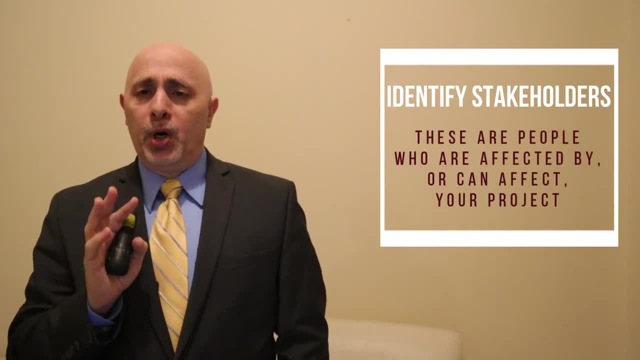 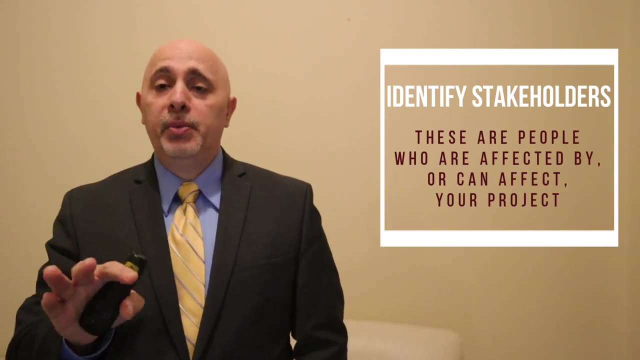 who has anything to do with this one project. They're either going to be positively or negatively affected by this one project, or they are going to. either they're probably going to be positively or negatively affecting your project. So either they're affected or 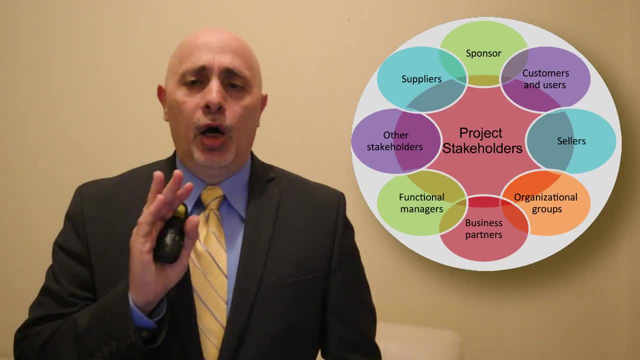 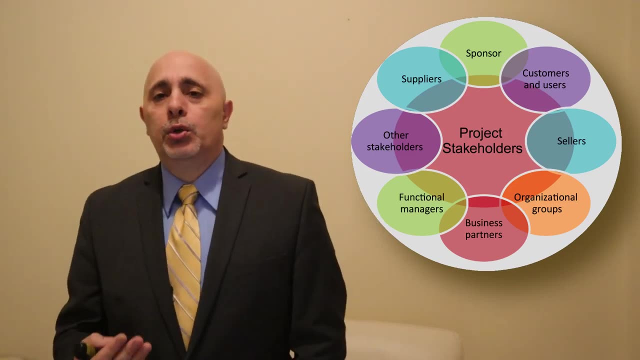 they can affect this one project. They could be a decision maker, a regulator, a contributor, a taxpayer. And that's the first step in your project. And the second step is to start with your technical resource: a department head, a supplier, anyone who is going to have anything to do. 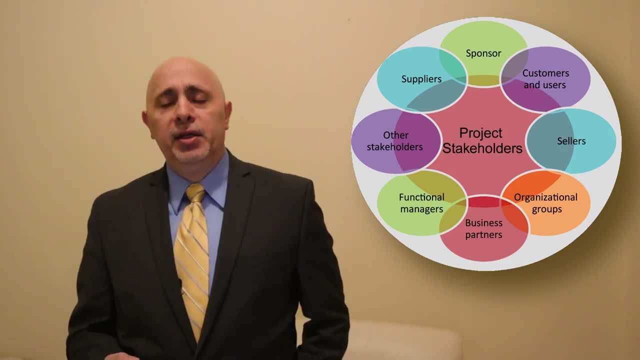 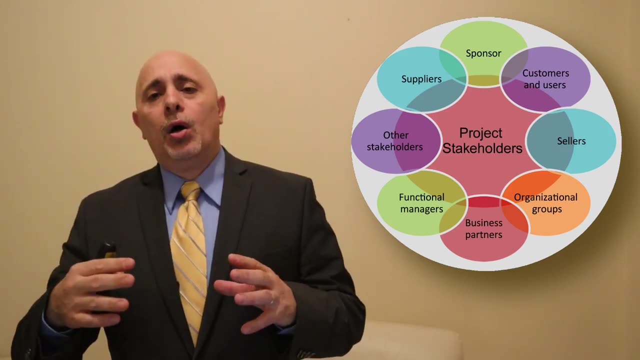 with this. one project is a stakeholder. You should try to identify your stakeholders from the inside out, from the people who are going to be working on developing the product of the project, all the way out to the organization and outside, to your customers or suppliers or representative of that. 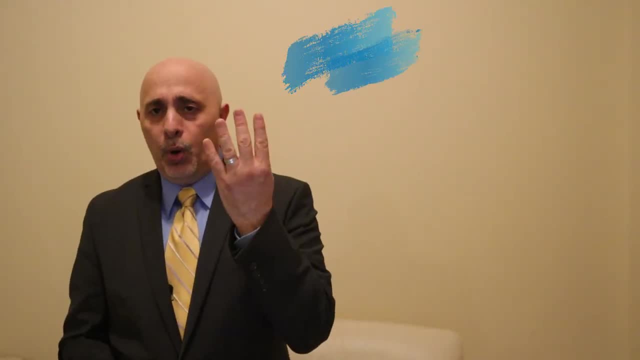 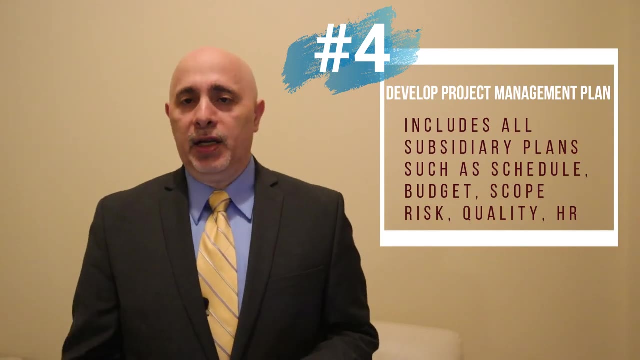 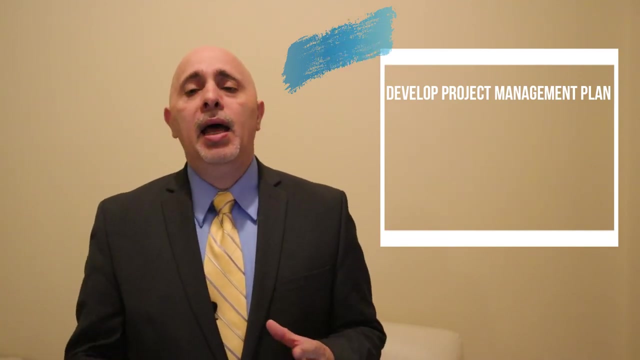 Once you've identified your stakeholders, go to step number four: Start preparing your project management plan. Guess what? Project management plans do not get developed in one day. They take time. You got to meet with all the different stakeholders and talk to them, understand how they feel. 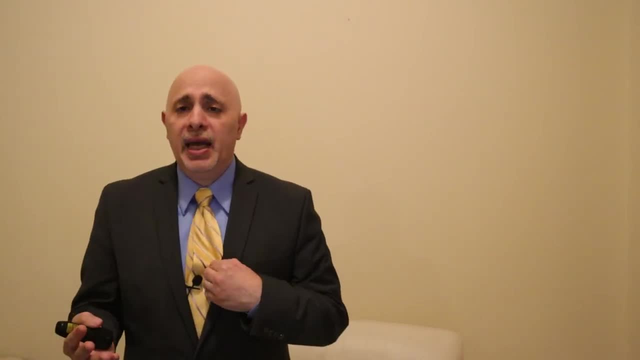 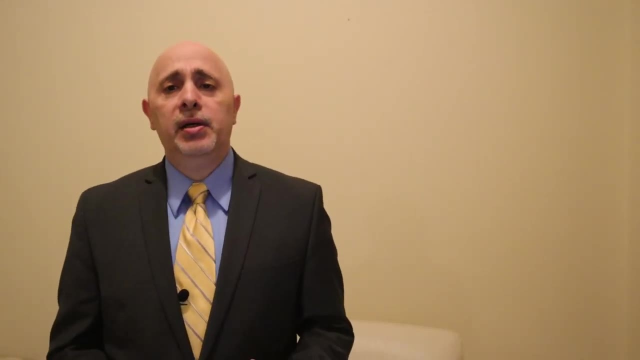 about the project, how they feel about the end product. Do they have anything to contribute? Are there any restrictions? Are there things you need to find out? Are there regulations you should consider? So project management plan means that you probably sometimes have to have a team. 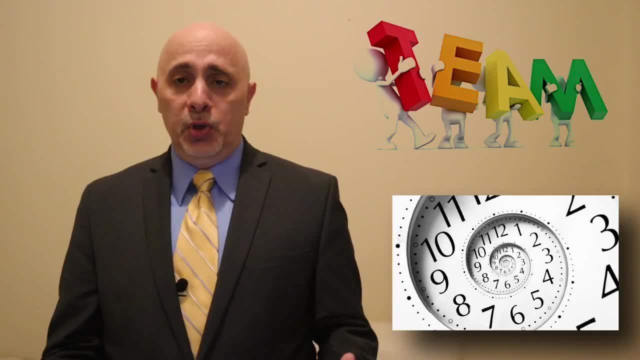 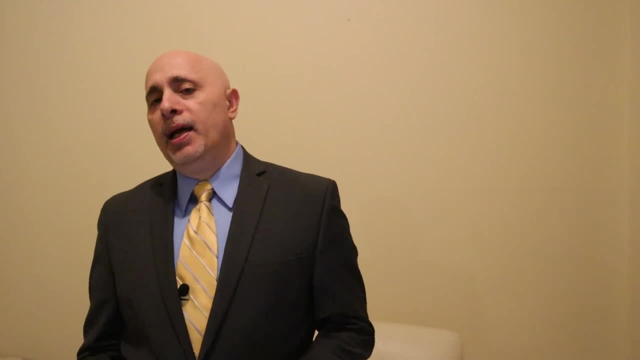 To help you with this and you have to spend a few days, after a few weeks, to get all the necessary details for you to put together a final plan. All right, So tell your boss the plan cannot be developed in one day and that you got to talk to everybody. 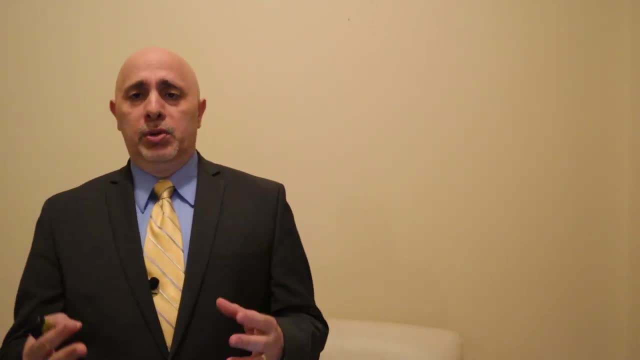 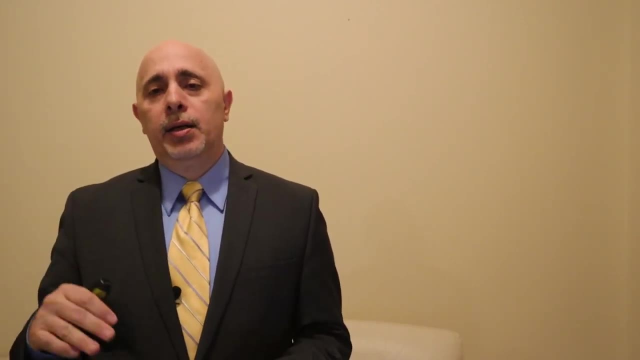 involved for you to be able to understand what's going to go into this one plan. So starting the plan is just one thing, and you're going to have a lot of subsidiary plans that are going to go into this project management plan. So now let's go into step number five. 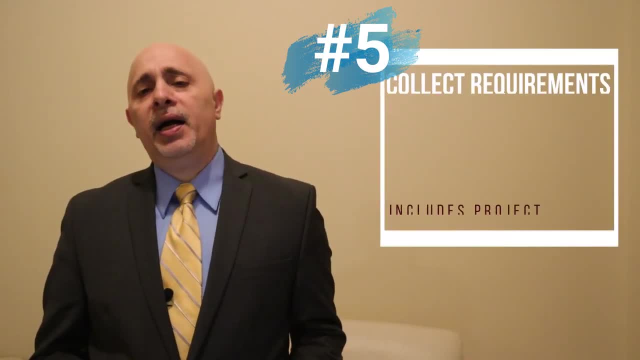 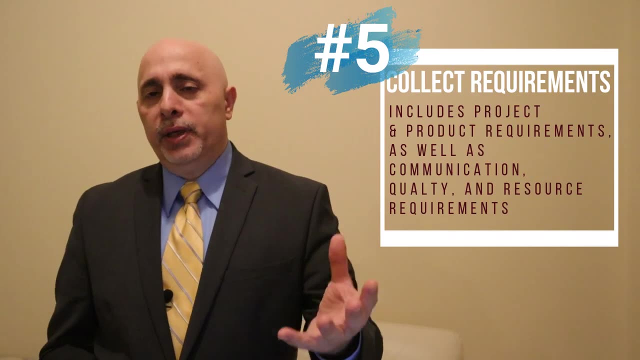 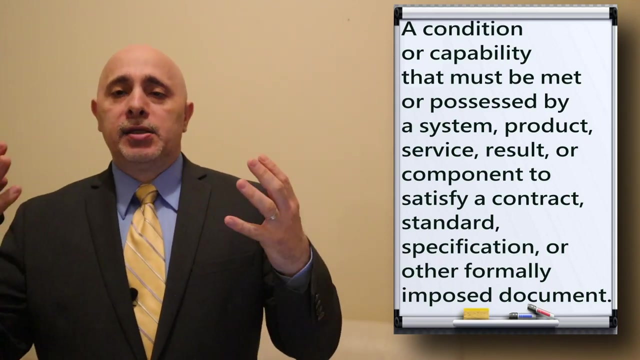 From your stakeholder list that you've identified. you need to start collecting requirements from those stakeholders. So a requirement, in case you're wondering, is either a condition or a capability. A condition means it's something that is put as a constraint on your project. 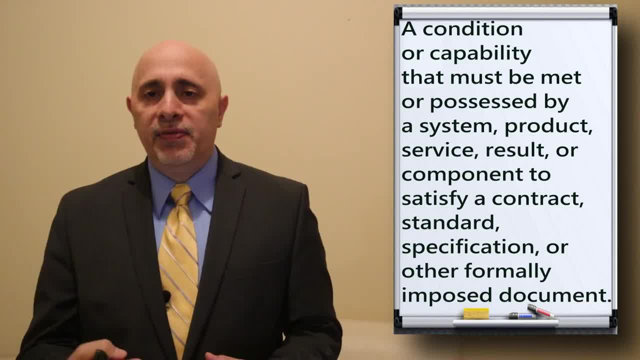 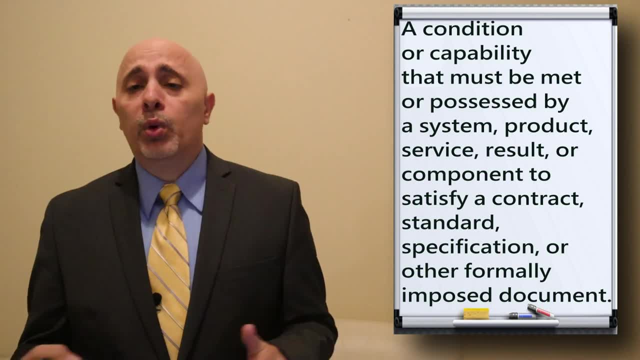 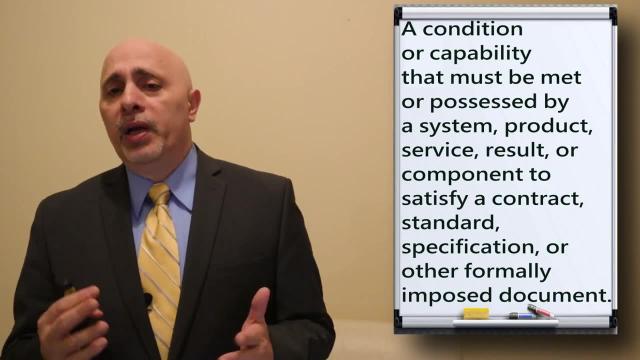 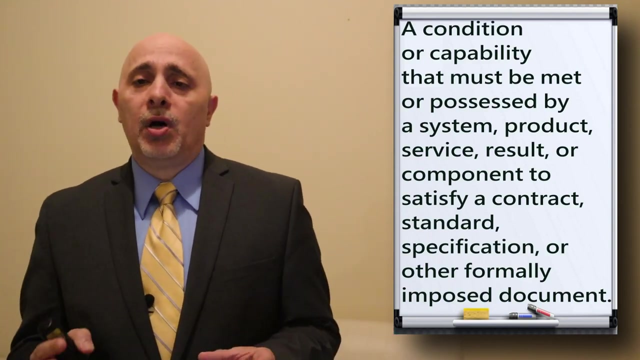 It's a beginning or an end date, a specific budget that you can't go over, a compliance requirement, For example, Working hours requirements, resource utilization requirements, whatever it is, language requirements. You know, language requirements can actually be a capability, but these conditions are. 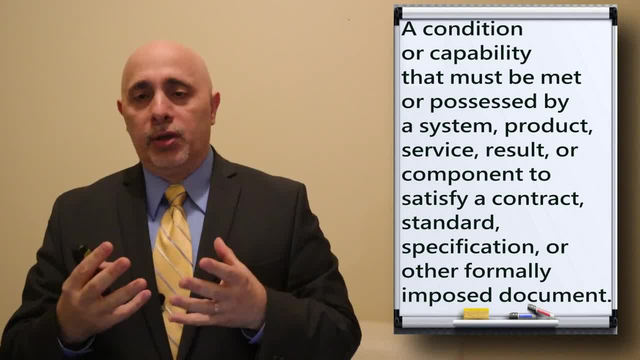 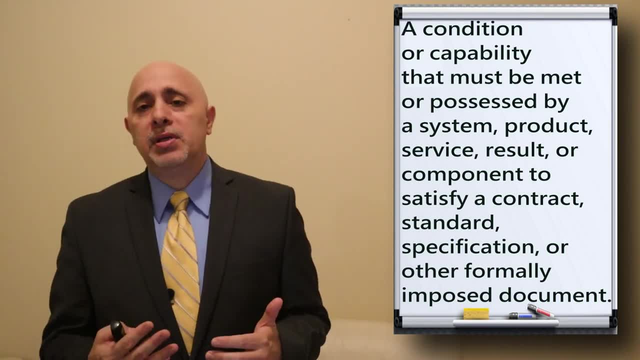 not going to be showing in the final product. in the looks of the product, What we'll show would be the capability and the capability, the capability requirements. Those are the ones that talk about what the product does right, So does it go. 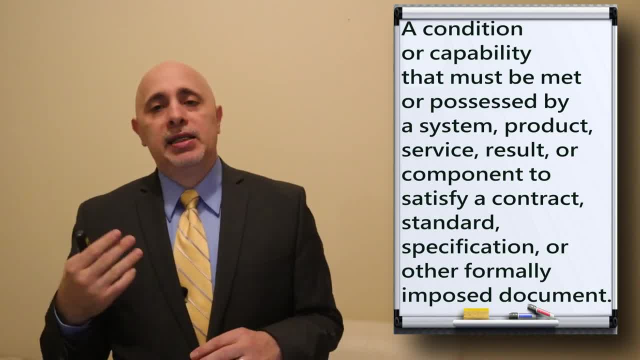 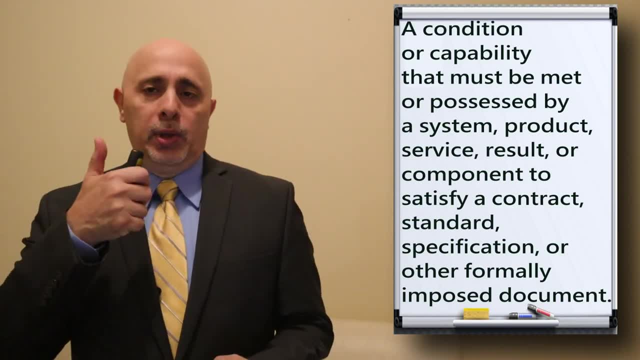 Does it make 100 rotations per minute? Is it eight feet tall? Is it made out of plastic? So these are the descriptive items of your final product. So you want the conditions and you want the capabilities, and these will be your requirements. 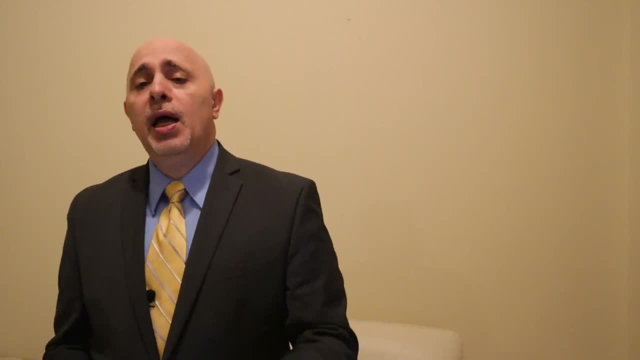 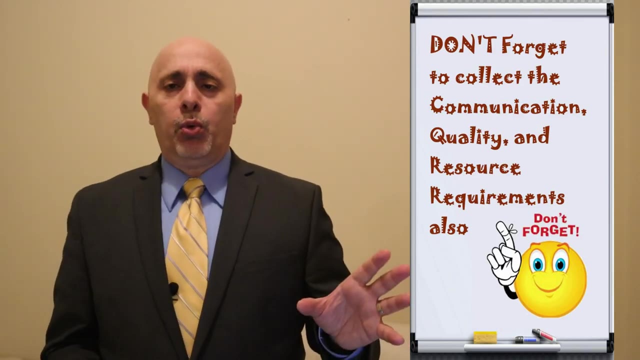 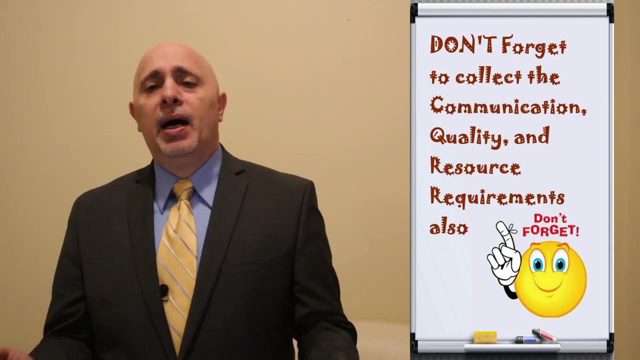 Once you've collected all of these requirements. oh, before we go too far, make sure you include quality and safety requirements and communication requirements and resource requirements. These are all part of the requirements, Don't Just The final product, the physical product. 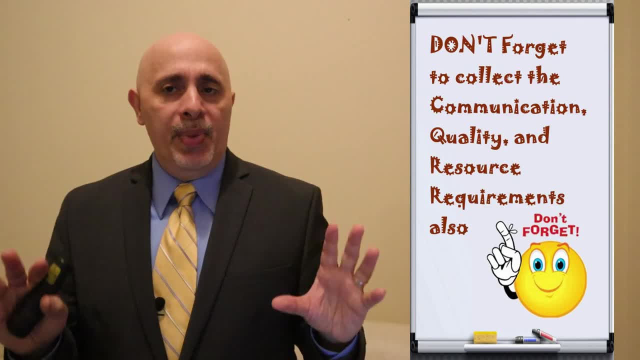 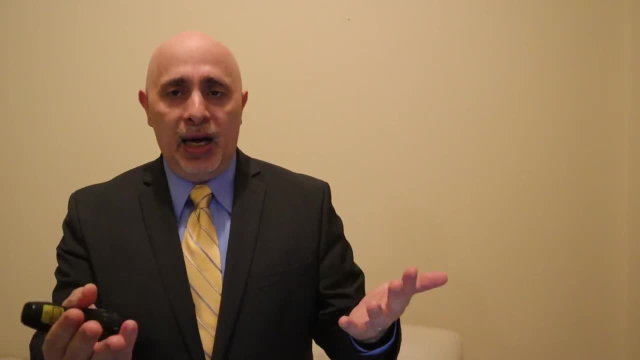 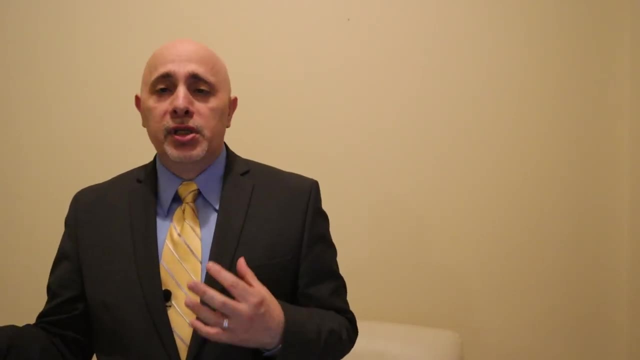 Think about what it takes- and these are what it takes- to actually manage this one project, And these are called project requirements. So we have the product requirements- That's what the product needs to have for specifications- And we have the project requirements, or project management requirements, which could be resources. 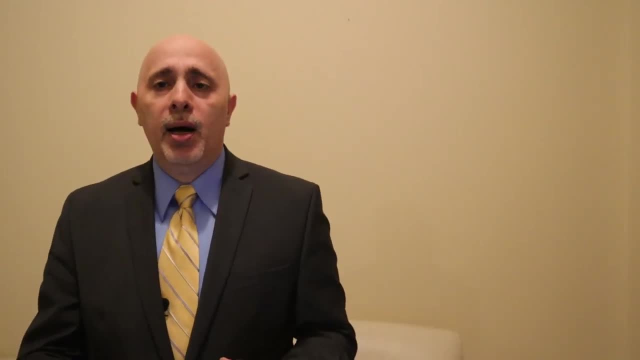 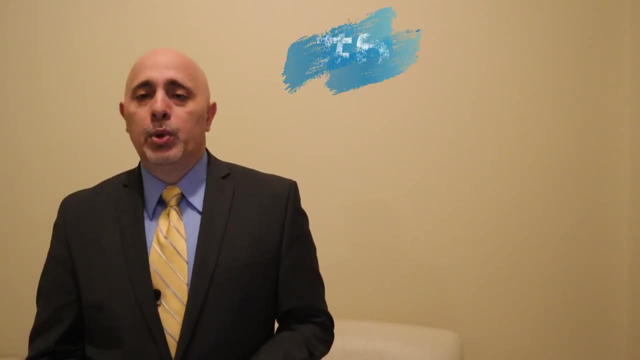 you need research that you have to do, meetings that you got to run, and so on. So these are your project management requirements. Collect all of these requirements And go to the next step, which is step number six, and that's to develop your scope statement. 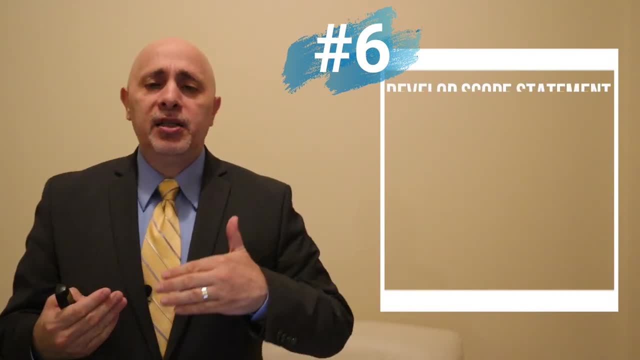 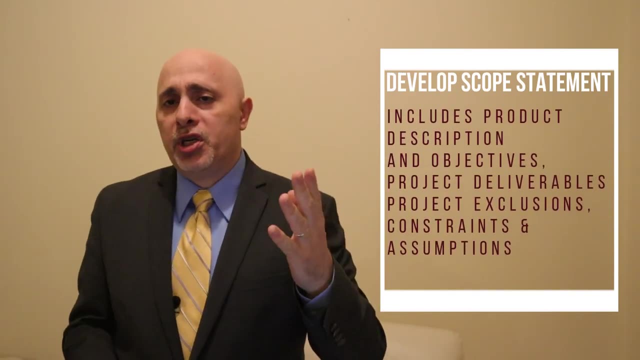 Your scope statement is an expansion or, let's say, an expanded project charter, It has a little bit more. So if you- basically if you took your project charter and you took your requirements and you added them together, you're going to get the scope statement. 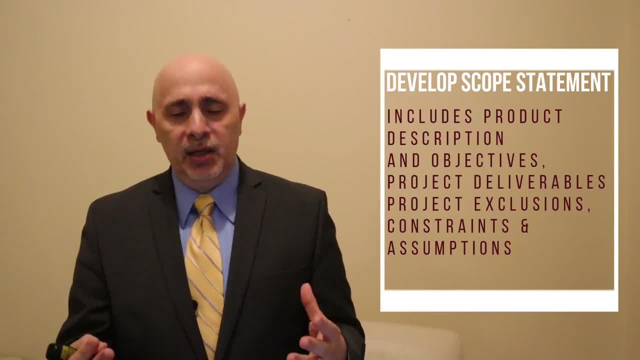 The scope statement talks about what the end product is that you're going to be delivering and what else you're delivering with that. Are you delivering? Are you delivering some coaching training? Are you delivering some technical manuals along with it? What are you going to hand over? 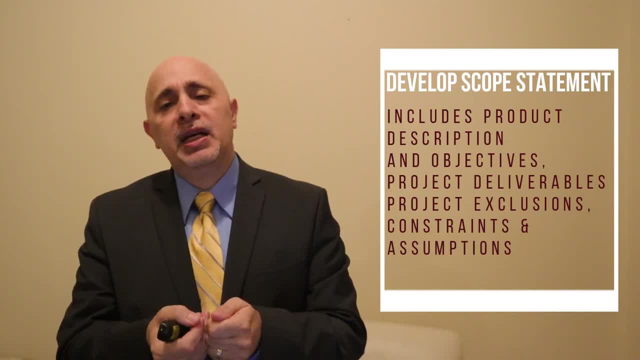 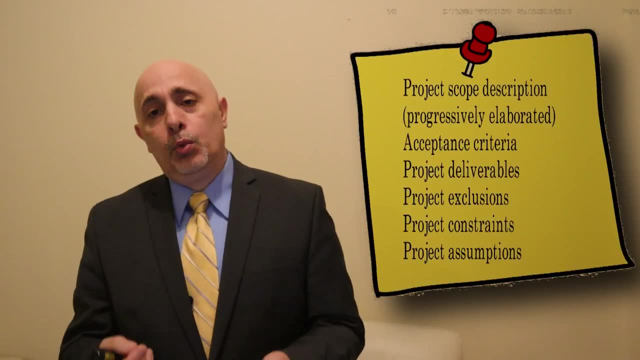 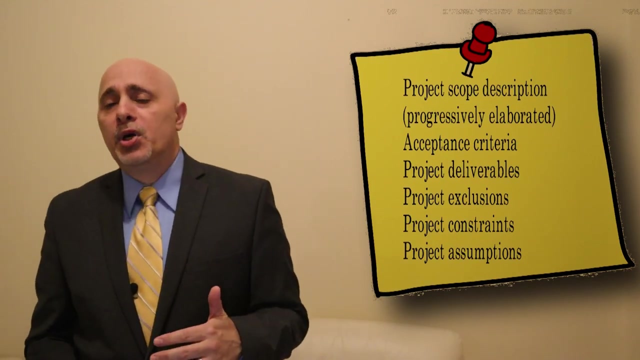 And those tend to be bulletized in the scope statement. The scope statement can be turned in with the list of requirements in order to make it more clear, And the scope statement. we also write what is excluded. If you think your customer or your sponsor is going to imagine some end product having, 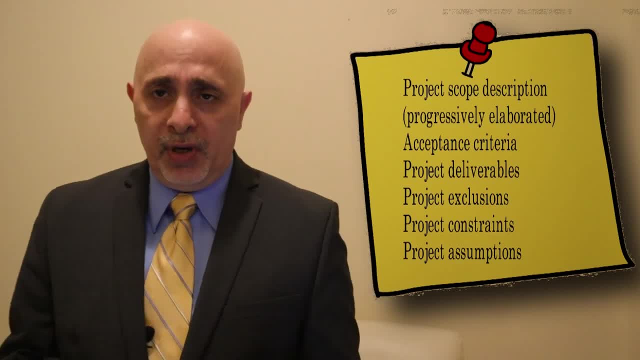 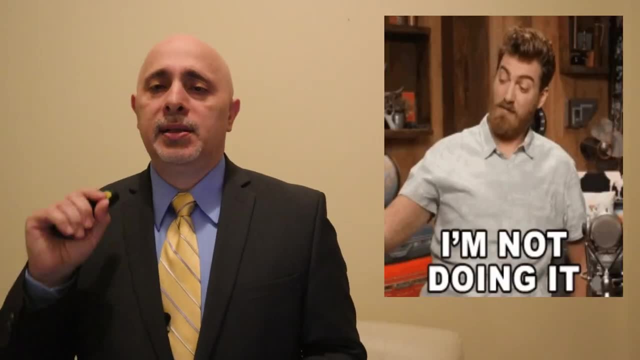 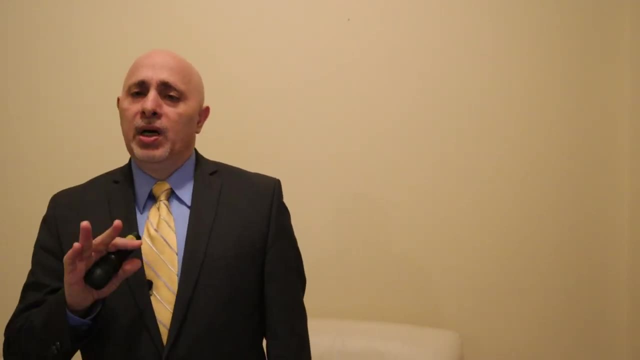 some additional specifications that you have not planned for, Then be very clear that these are not state them in the exclusions, that these are not part of the scope deliverables. So that's your scope statement and that's step number six. Once you have your scope statement, and let's say, you review it with your sponsor and your 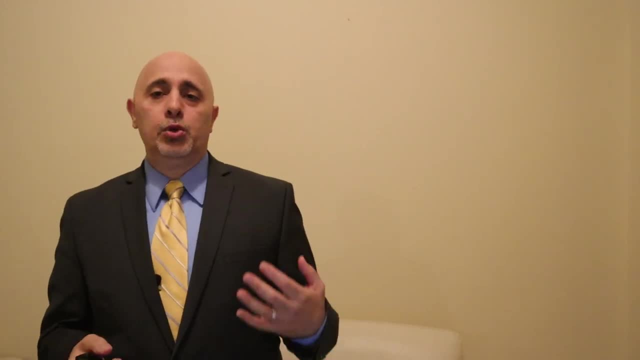 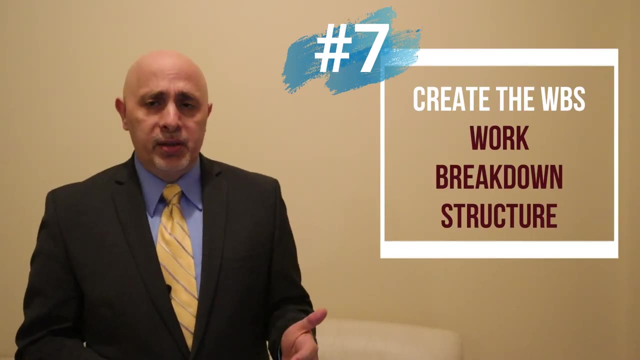 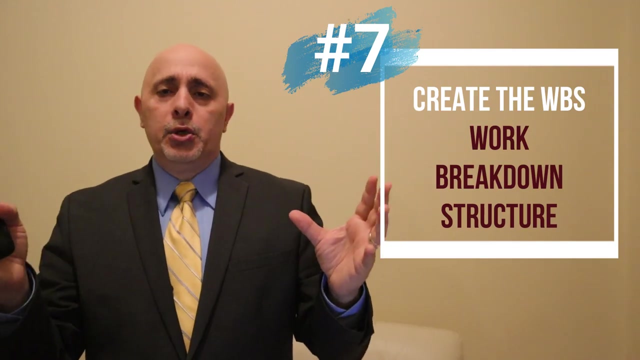 sponsor is okay with it. it is time to plan out how this is going to be executed, And that takes us to step number seven, which is to create your work breakdown structure, The work breakdown structure, called sometimes just the WBS. It's similar to an organizational chart. 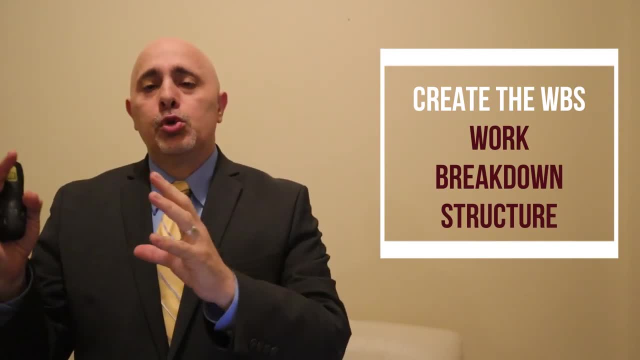 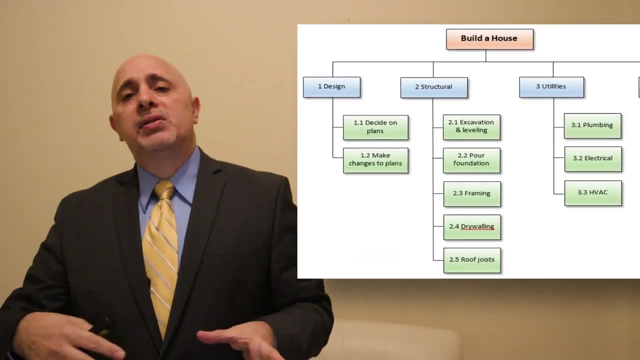 You're taking all of the work and you're breaking it down into smaller pieces. So you could break it down by the nature of the work. A WBS represents all of the work that is going to be delivered, but it is broken down into. 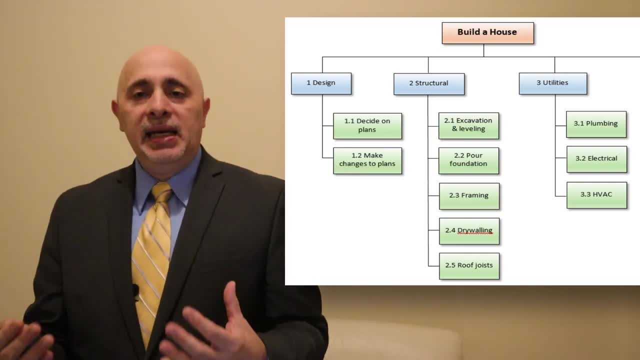 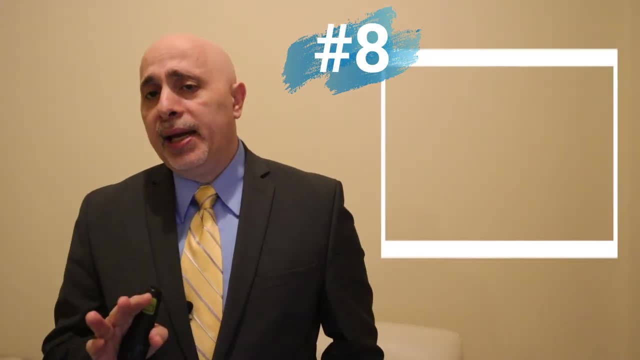 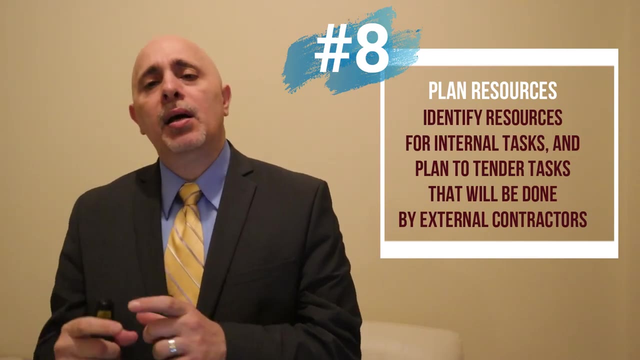 smaller, tinier pieces. that makes it easier to manage. So after you do your WBS, you go to step number eight, Step, Step, Step, For step number eight is to look for what resources will be required for every one of these WBS work packages. 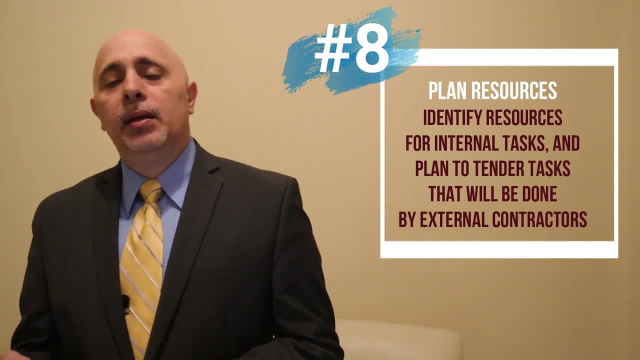 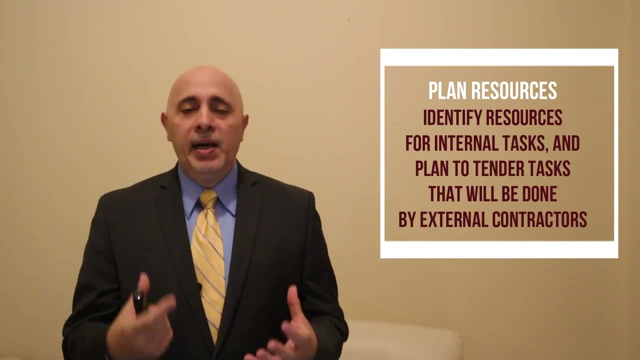 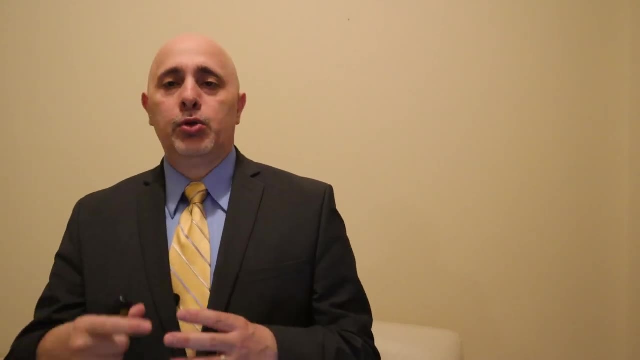 Underneath, there is going to be activities that will need to be done to deliver that one package. So if your team is going to be working on that one package, what activities are they going to be doing? So typically, what I would do, what most projects have to do, is that every piece is assigned. 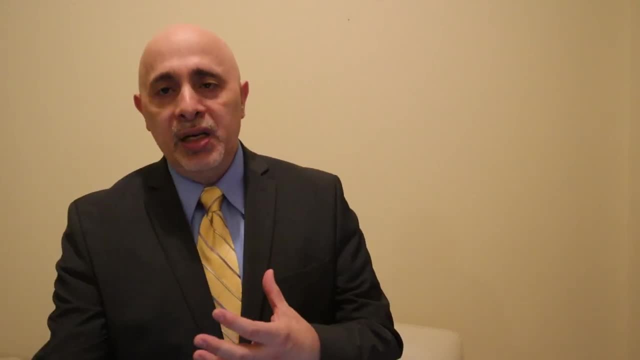 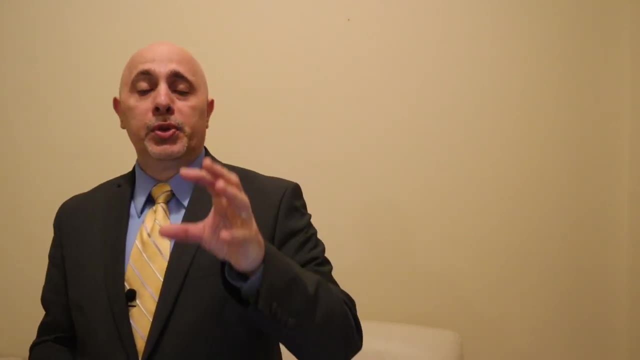 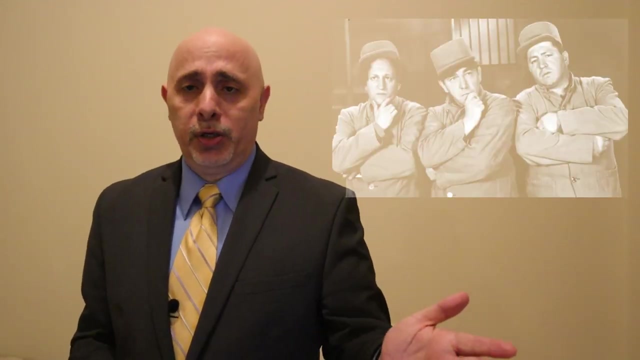 to a team lead who then has their own resources or team that would be doing the activities for that one task. and, by the way, you probably would have to go to department heads and negotiate for these resources and make sure they give you the better ones, not the ones that were happy to just dump on you right, and then you know, probably count them. 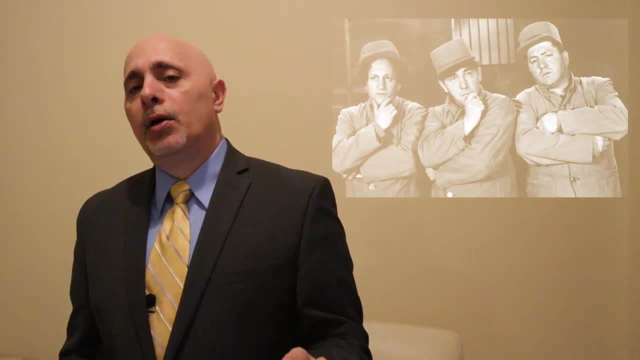 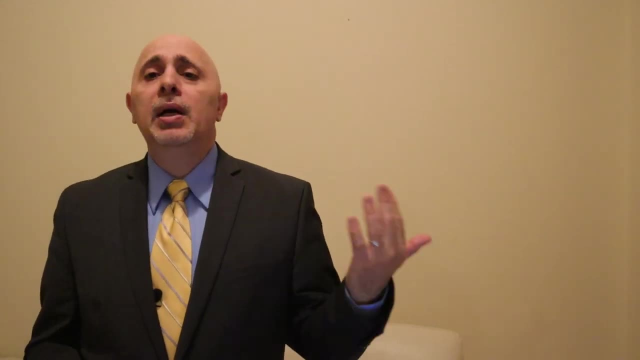 you know, as a relief budget wise, make sure you get all the good people and ask for how many hours they can allocate to your project, so that you know from the beginning whether you need to get some additional contractors on the project or not. if it's a contractor, then the contractor. 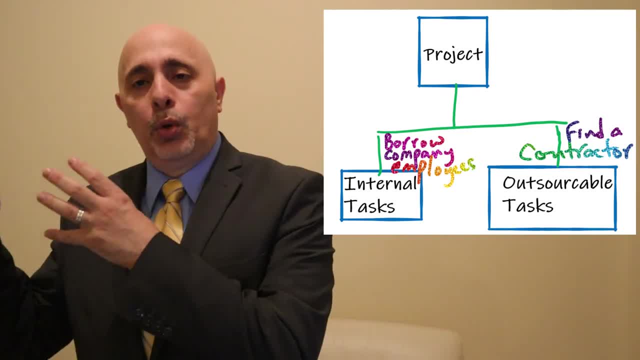 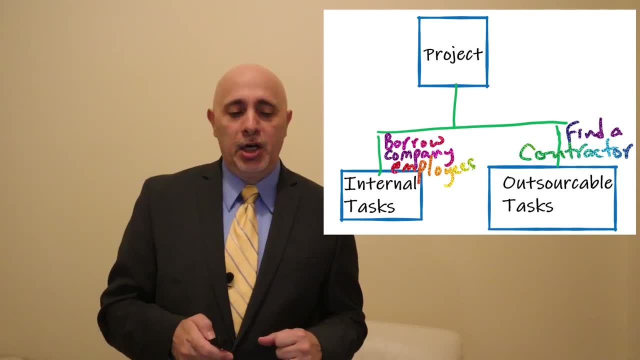 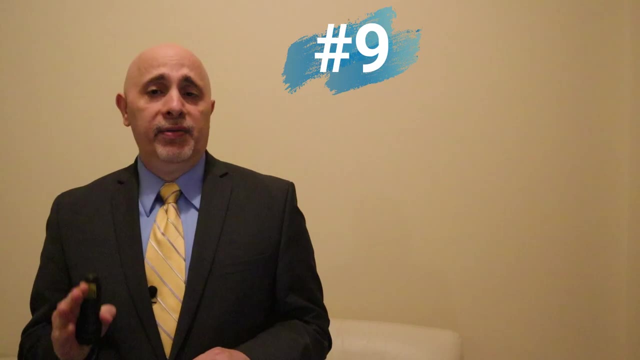 will tell you what sorts of activities they will be doing. they have their own team or resources that will be working on it. so step number eight looks at the resource requirements for that one project. so once you figure your resources out, then let's go to step number nine. step number nine is to develop your project schedule. now, project schedules are pretty. 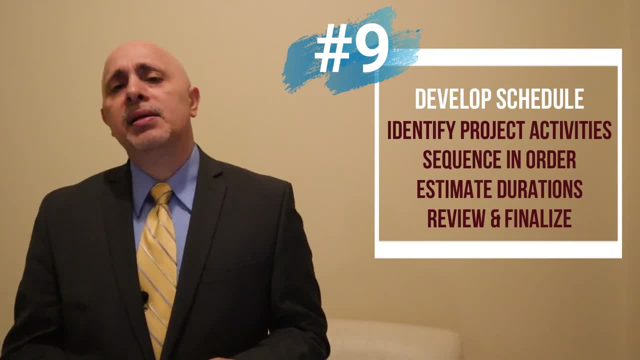 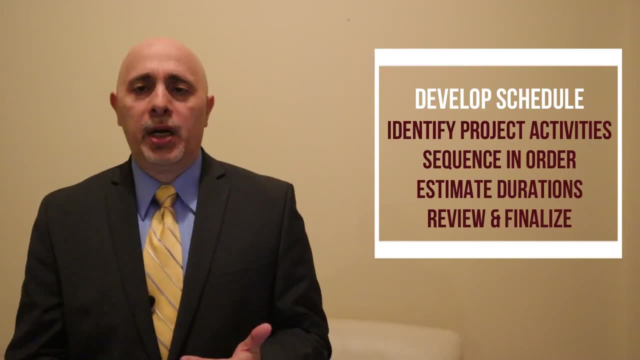 common and you know i've seen a lot of people who have been doing it for a long time and they varieties of these. the very, very basic form can be developed in Excel, but Excel isn't as versatile and does not allow you to make changes easily and doesn't. 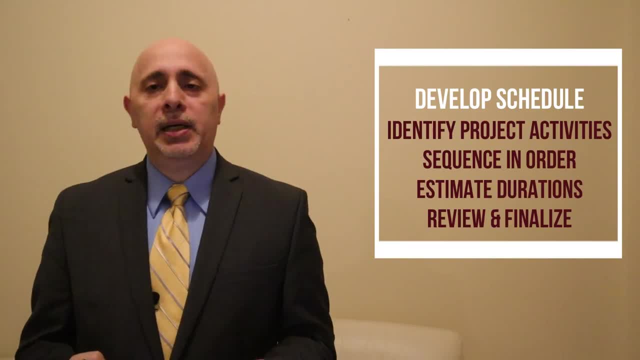 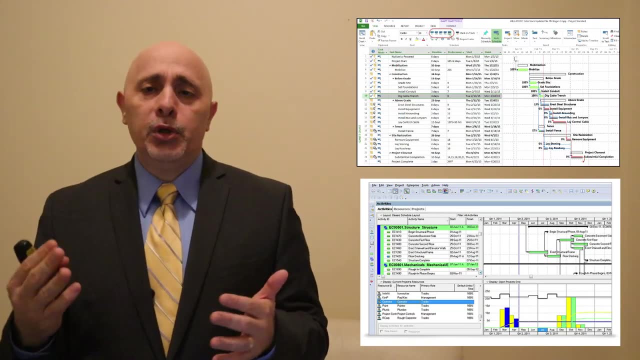 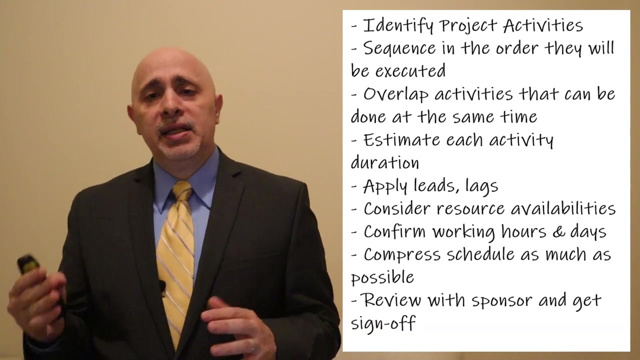 show the connections between activities. the best way to do it is using thing you know, software like Microsoft Project or primavera, and this way you can use bar charts. you may want to look at a different video on how to develop schedules, but you got to develop your schedule by taking all the activities. 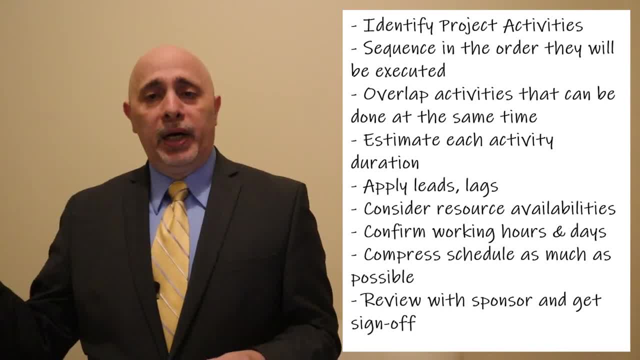 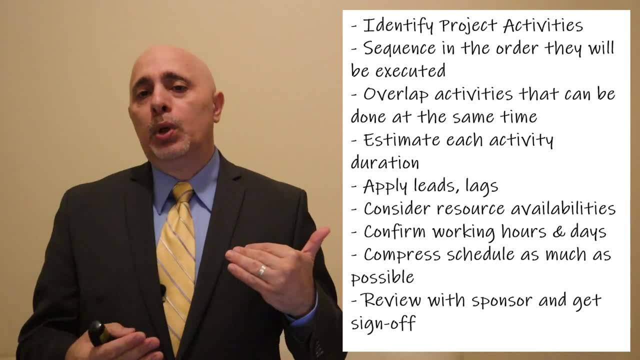 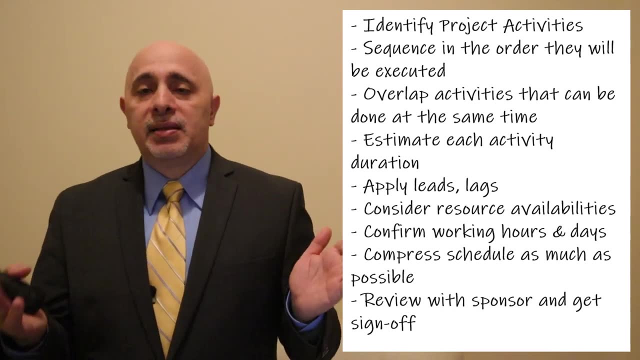 that were previously identified by your team or by the contractor, and try to sequence them back-to-back with durations, with dependencies. understand which one needs to wait for the other. understand which activity can run at the same time as the other. validate the time estimate that they're using for these. 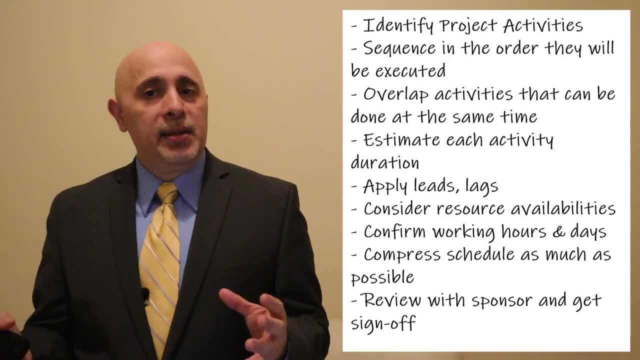 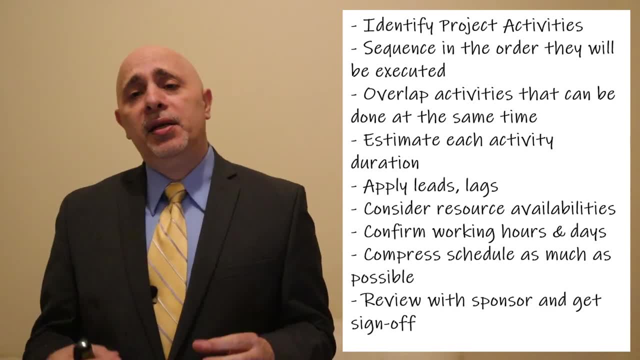 ask them. you know the basis for their estimates. where did they get them? is it based on experience or is it based on being, you know, maybe pessimistic? but finally, if you have any questions, please feel free to reach out to me at the end of the video and I will be happy to answer them so you can find out where. 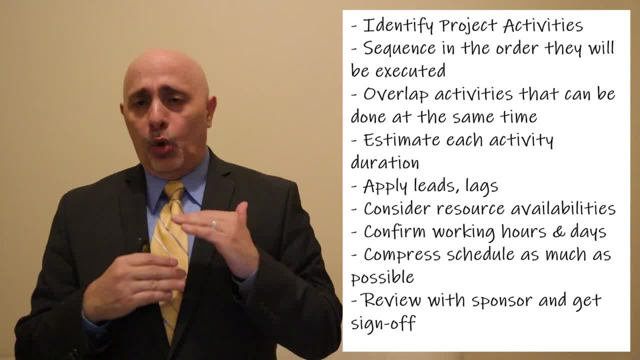 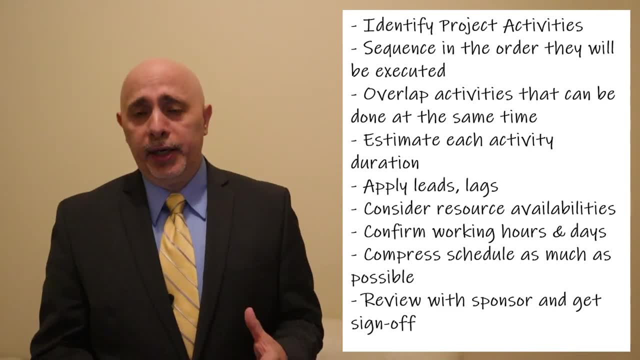 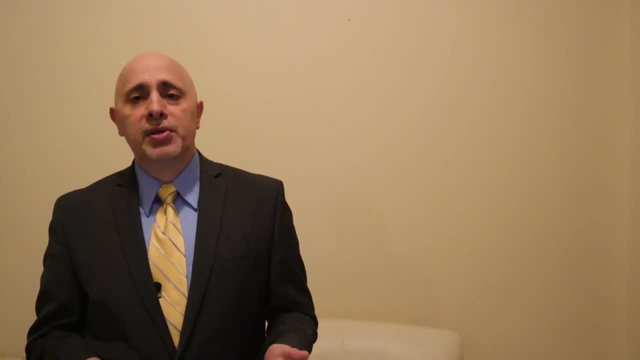 the estimates are coming from, and try to develop, put all the activities and proper sequencing overlap- the ones that you can- so they can run at the same time, and then that would also clarify the resources that you're going to require. so once we've identified how long the project takes, now we need to review it. 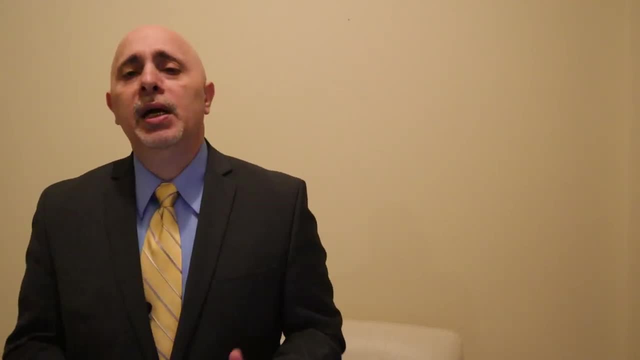 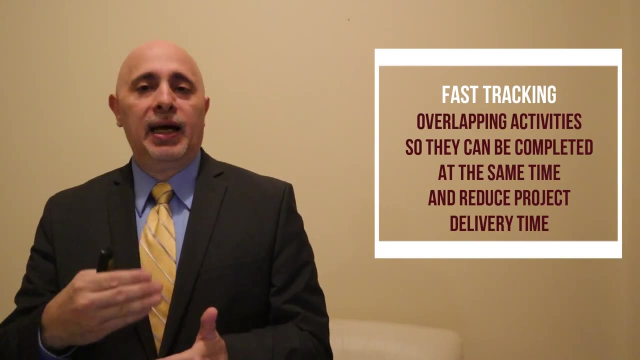 with the sponsor and make sure they're fine with it. a lot of times, they will ask you to simplify it or make it shorter, and so what you have to do is look for opportunities for you to overlap, or what we call fast track, to track fast track. some of these activities overlap them. run them at the 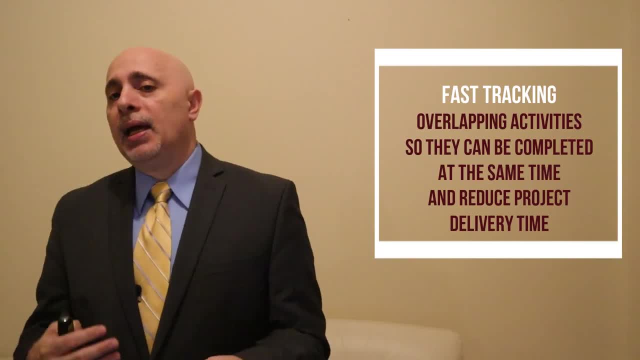 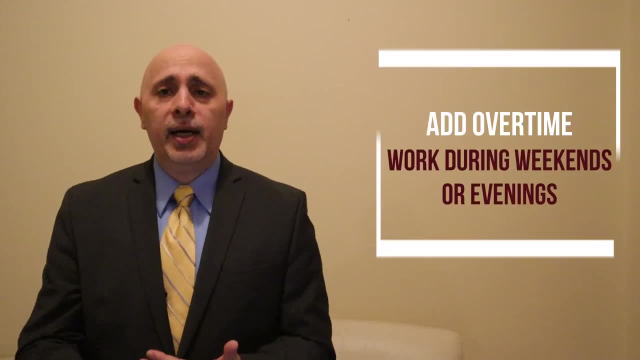 same time, that's going to increase your risk a little bit. and then look at adding, maybe, resources in some places which we call crashing, and or maybe look at the working hours over time and so on. or maybe look at, you know, building efficiency in the team or using better tools for them to get things done, and 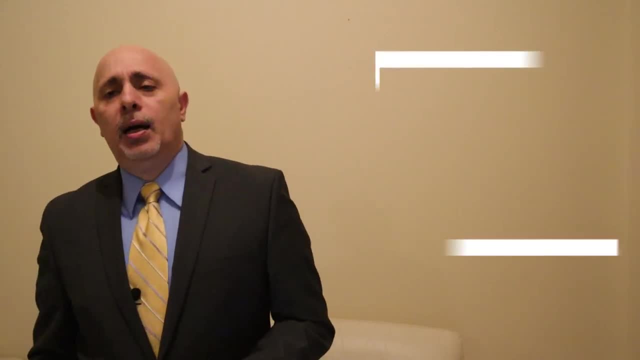 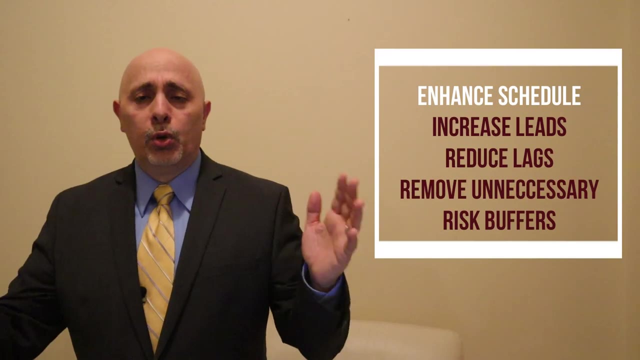 that's going to speed up your project, all right. look at putting leads where you can have something start and not really wait for something else to be finished. if you can, right. if you can't wait for something else to be finished, and if there are lags or waiting periods that are unnecessary, you remove. 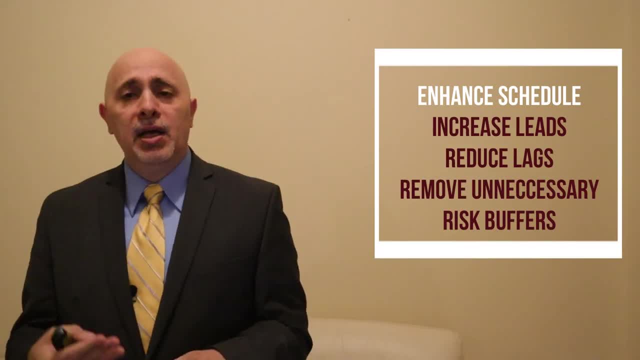 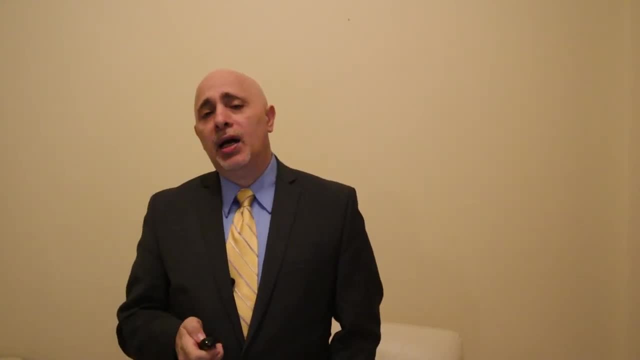 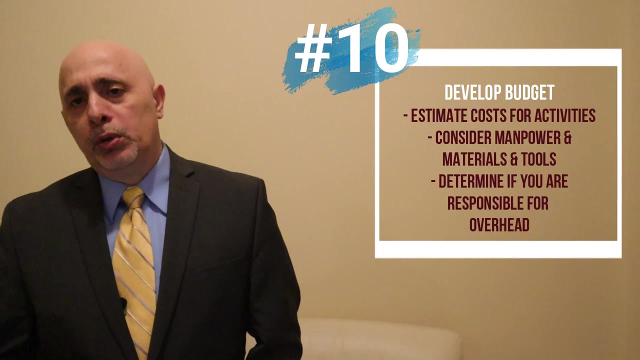 those, remove any buffers or any padding you've put for, you know, for risk into that project, so that you can reduce the duration of that one project. once you have a schedule that your boss is okay with, then it's time to develop the project budget. you do know the resources that we are working on it. you do know. 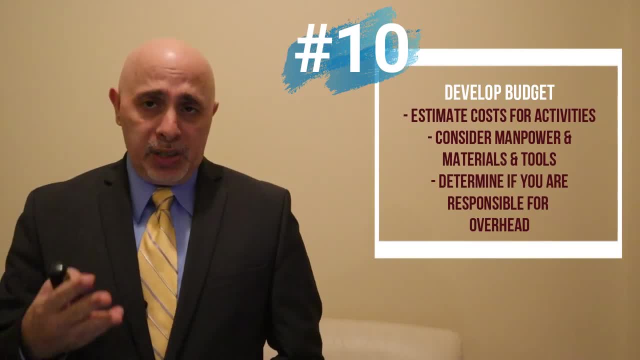 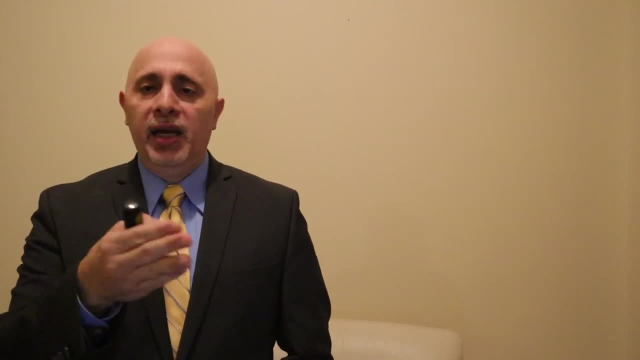 the resources will tell you what sorts of materials they'll be using on the project. all you need is cost estimates for the resources and for the materials and you can have your budget. you can even figure out what you'll be spending weekly, monthly, quarterly if you want, and that's. 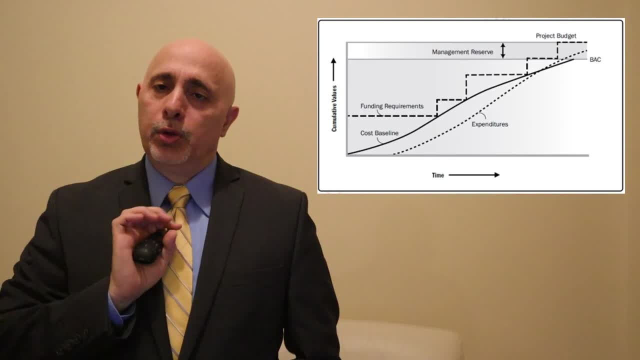 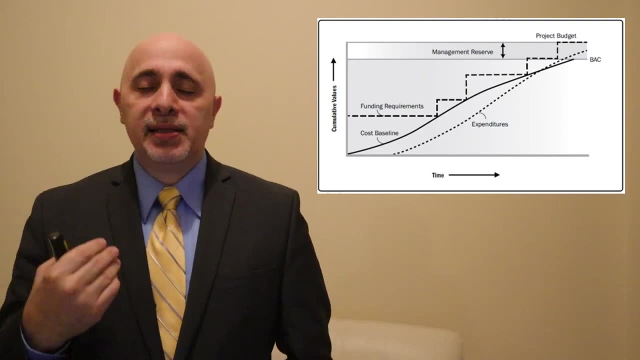 going to help you develop your cash flow analysis. it's mostly going to be cash going out and but you're going to figure out what it is that you need for money to fund this one project and you can ask. you can develop a funding schedule for your management so they know how much to fund you every quarter or every month, if 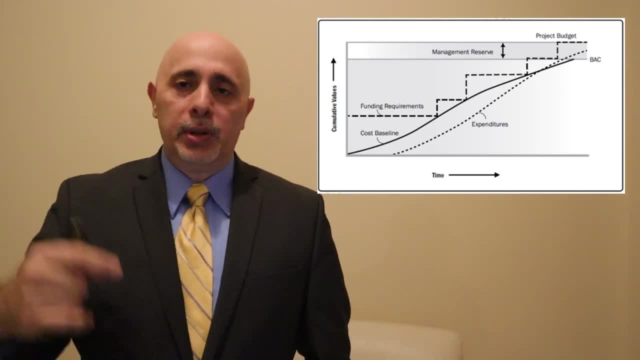 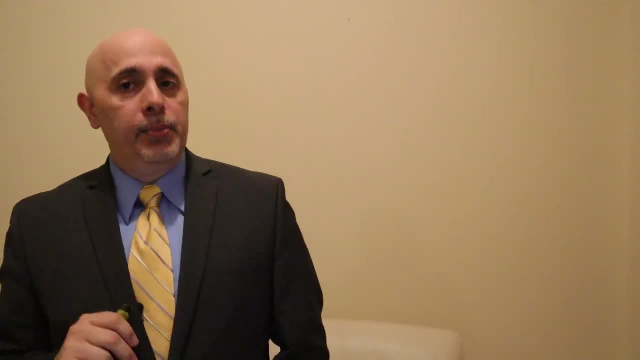 that's how they're going to be funding the project and they would know what to expect going down the line. all right, the schedule and the budget and the scope, the requirements, all these that we've talked about- can later be used to monitor your project and see how your 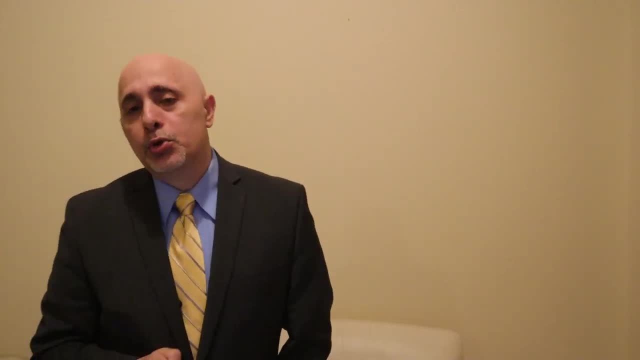 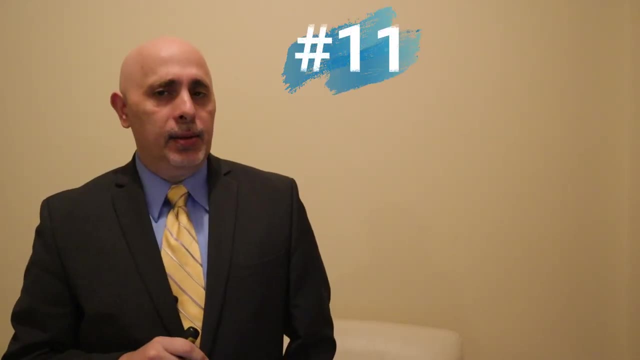 project is going. having a good plan means you have something you can use to monitor your project once you have your budget. that was step number 10. now let's go to step number 11. step number 11 has to do with asking yourself what could go. 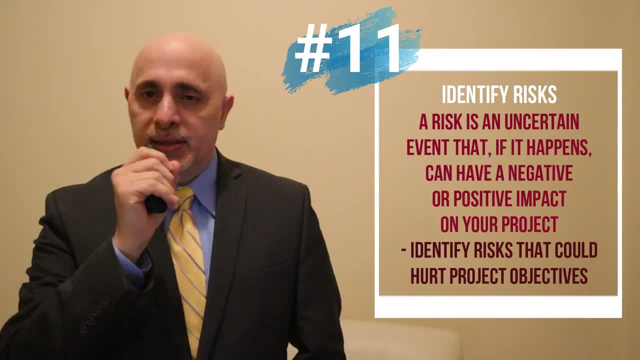 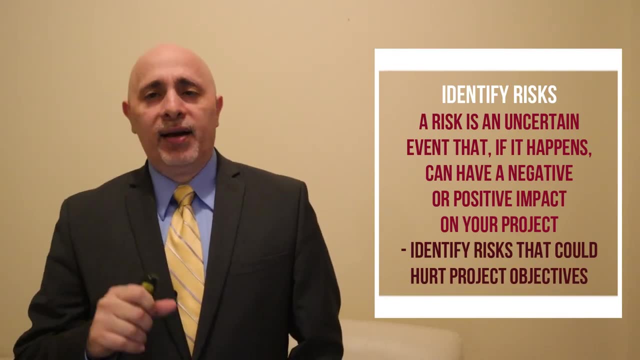 wrong on this one project? now we're talking about risks. what are the risks in your project? what could go wrong on your project with all these plans that we have? we've identified the stakeholders and we know some of them can be troublesome. we've identified requirements. we've put 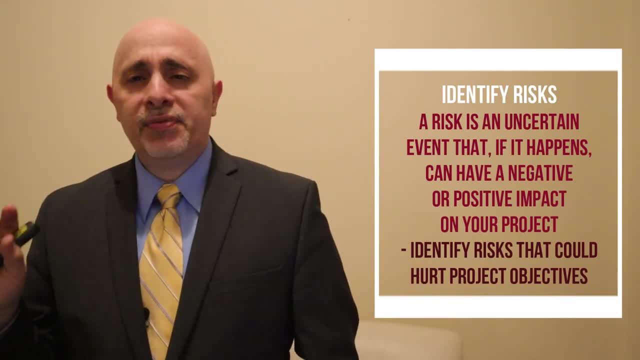 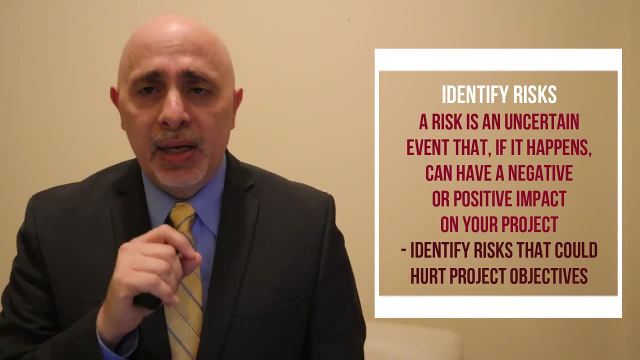 together a scope statement. we've, you know, created work packages. we've started thinking about outsourcing some of the work. we have a schedule. we know the resources that we're working on it. we know the budgets that have been estimated. what can go wrong on that one project? all right, so sit with your team and try to. 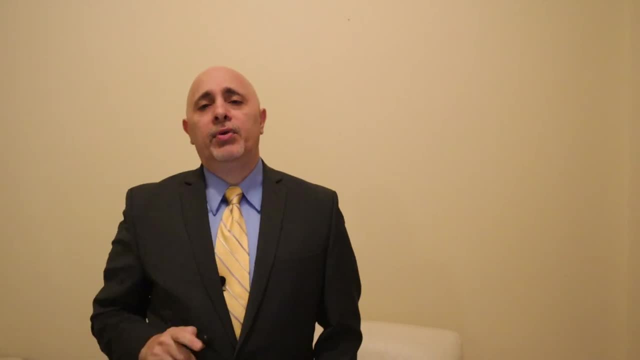 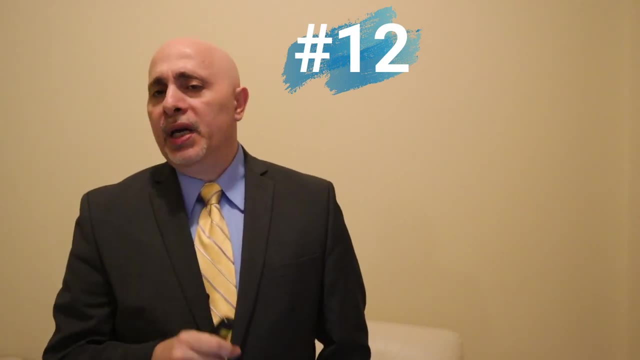 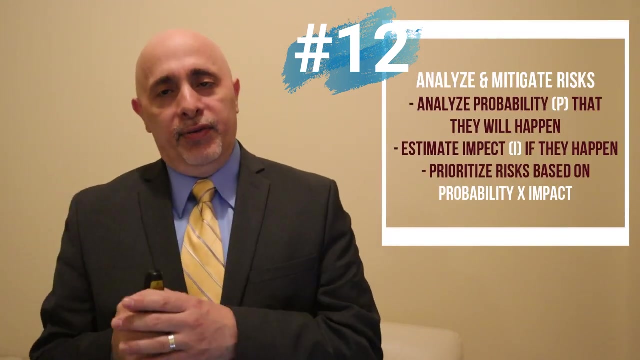 figure out what could go wrong and then, once you have a list of all the things that could go wrong- the risks- then go to step number 12: mitigate those risks. what does it mean to mitigate? find ways to reduce the chance that a risk can happen or to reduce the effect if the risk actually happens. look at the probability. 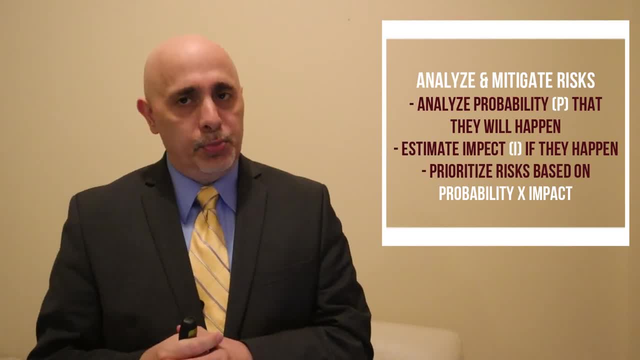 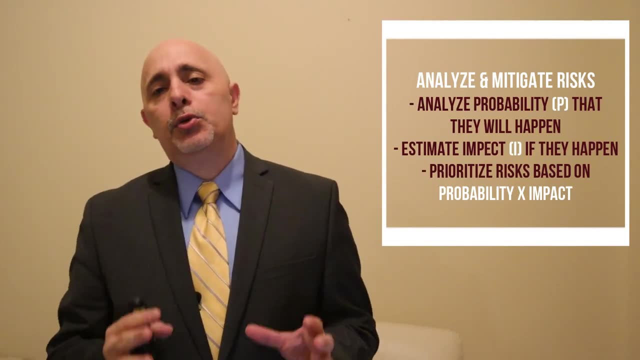 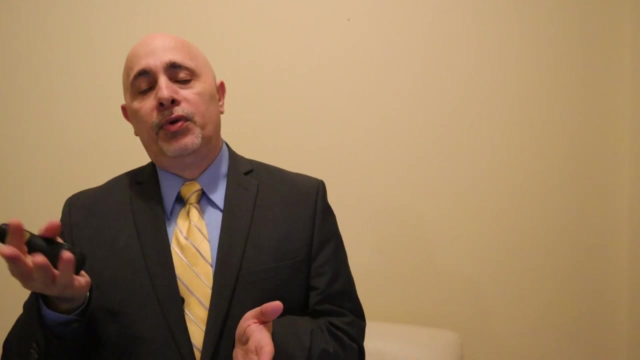 that a risk can happen and the impact it would have on your project objectives. if it's not going to affect your project objectives, it is not a risk, OK. so you need to have a clear understanding of what the project objectives are and then looking for the things that could affect them and look for ways to mitigate them. there are four. 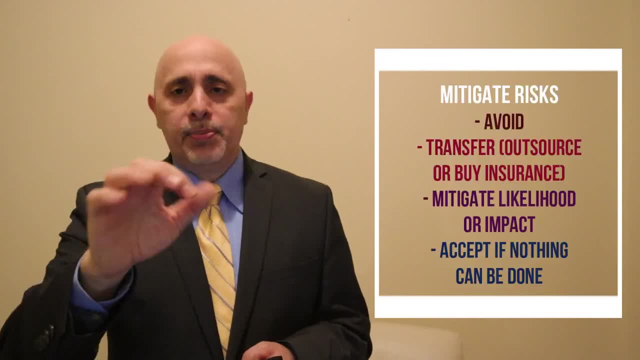 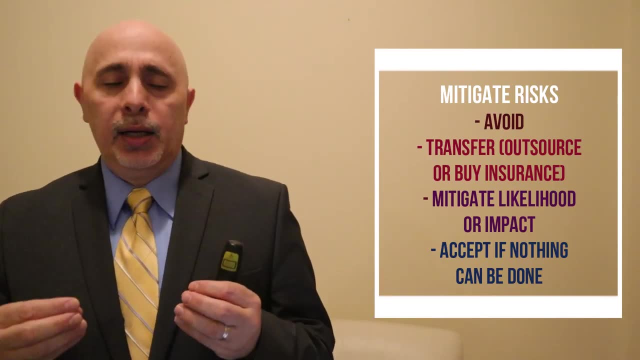 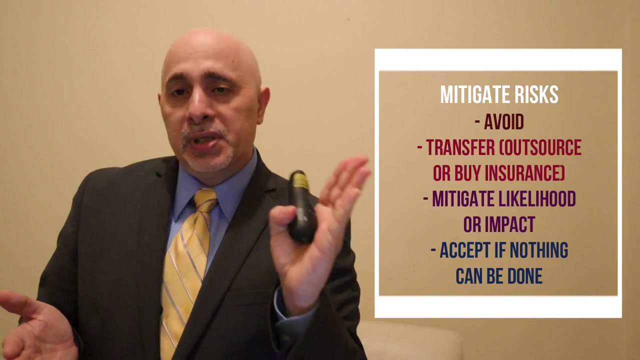 ways to mitigate risks right, you could avoid the risk by taking it out from your project. so a certain software presents a problem for you. you think it might not be. it might not integrate. well, so take that software out. and now you've avoided that one risk. but you might introduce a secondary risk that way. 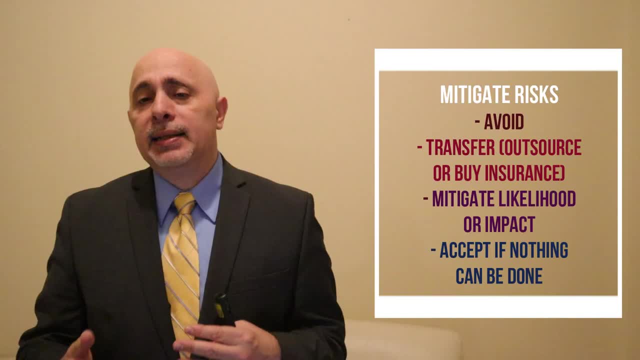 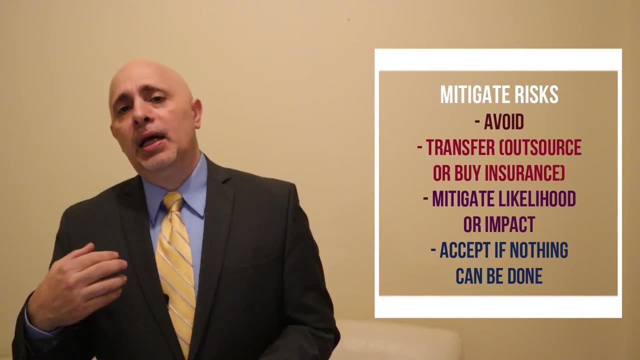 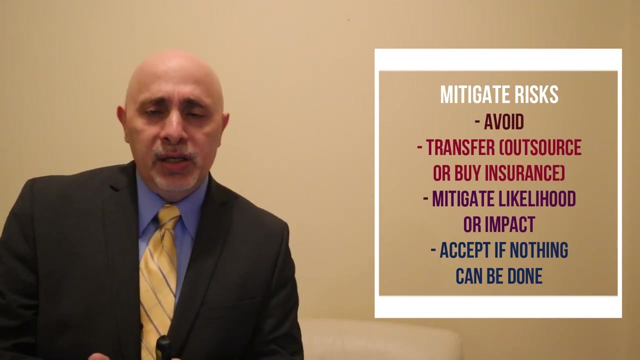 right. If you can't avoid the risk, then look at transferring the risk, which means outsourcing or buying insurance, if that's a possibility. If you can't transfer the risk, then look at mitigating the risk or reducing the probability or impact of the risk happening, adding additional resources. 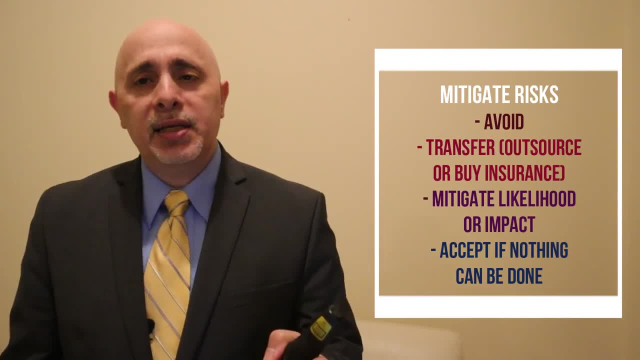 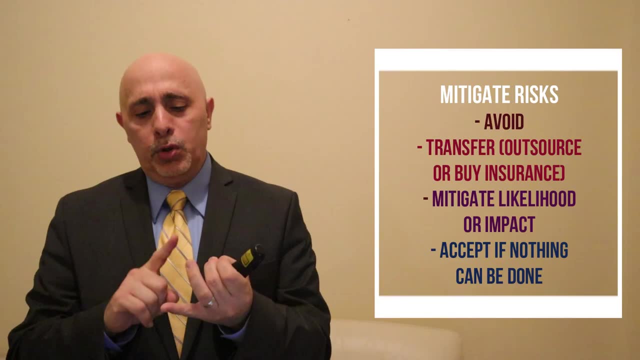 taking additional training, double checking, improving your quality processes. that will mitigate the risk a little bit. but that's all going to come at a cost. Let's say you could not avoid, you could not transfer, you could not mitigate the risk. then you may want to consider: 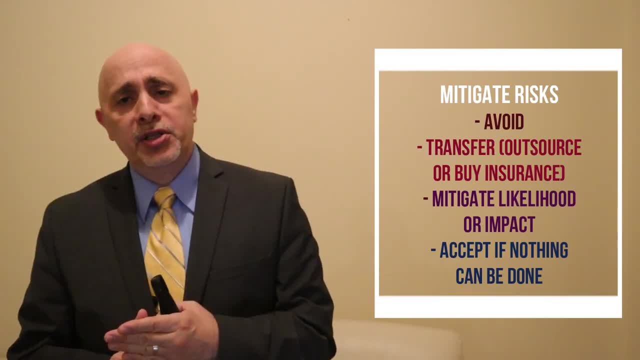 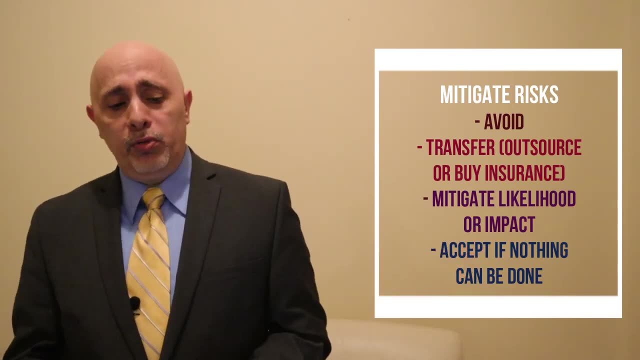 accepting the risk. all right, You could accept and put a budget. you could accept- you know a contingency budget- or you could accept and do nothing about it because there's nothing you can really do about the risk. So that was step number 12, you developing your mitigation plan. Step 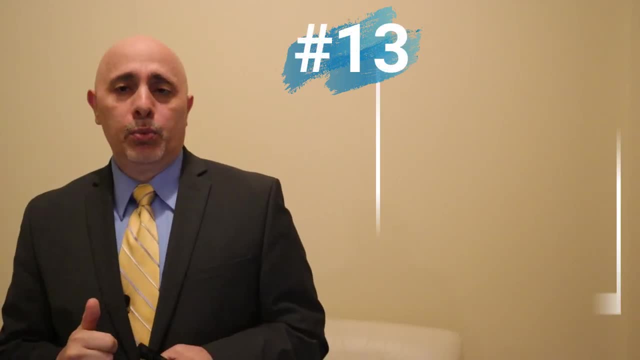 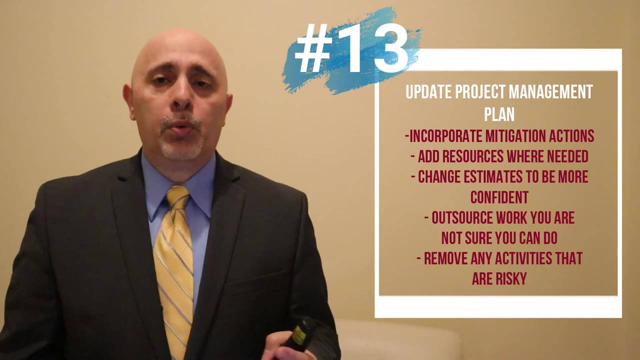 number 13 is to update your project management plan with all these mitigation actions. You want to make your project management plan, your scope, your budget, your schedule, your requirements. you want to make them more likely to succeed, And so you're going to change. 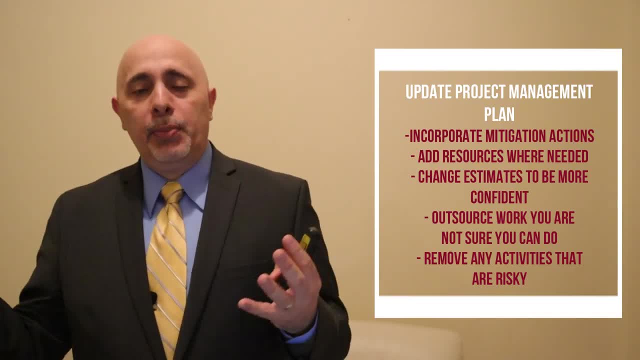 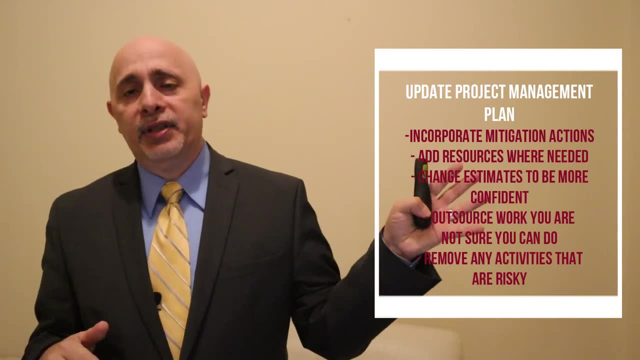 them using the mitigation actions that you came up with. So if you thought you're going to eliminate some software from the program, fine, eliminate it Now. your new plan does not have it. If you thought you're going to have additional two resources, or maybe someone who's more senior, 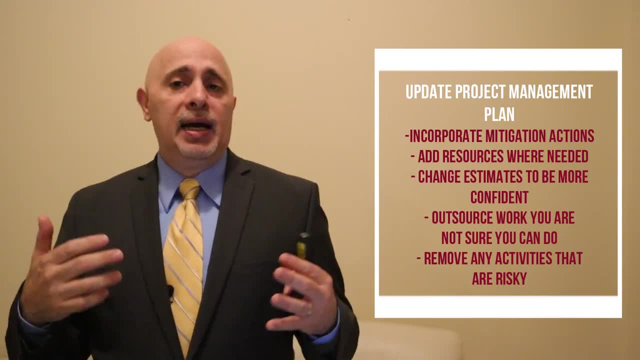 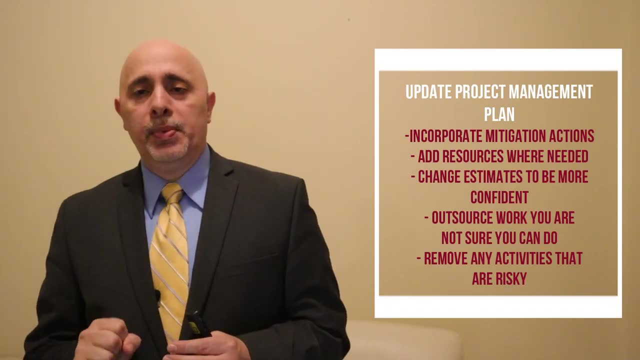 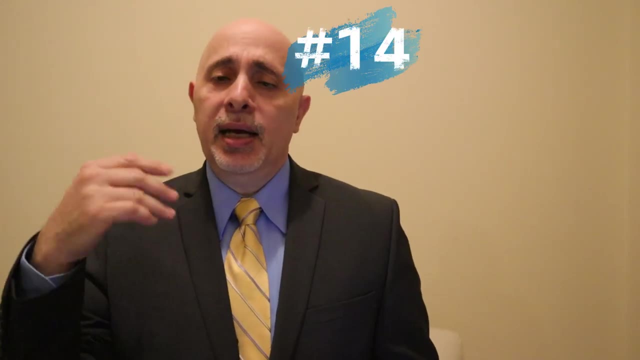 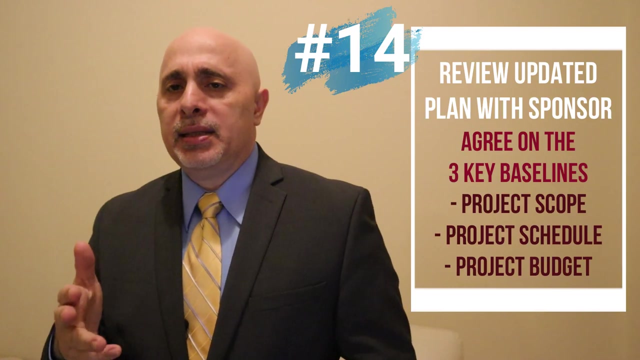 on your project, then do that Now. your project is safer. It has someone who's more skilled and can do the project for you. So your mitigation actions- they're not necessarily the solution- or considered joining the additional 4G system or systems for 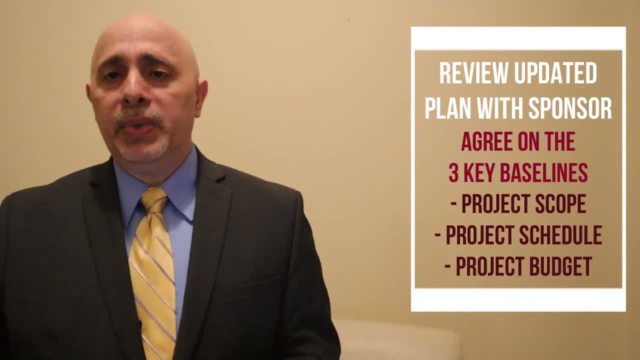 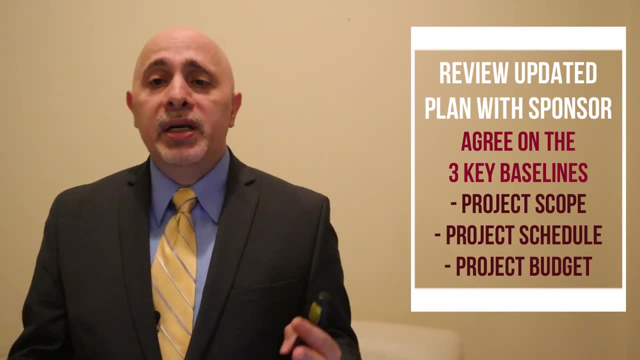 you. You need to be added into your project management plan and modified. And once you have the modified project management plan, we go to the final step, step number 14: sit with your boss and tell them what the reason, who the resources will be, what sort of a schedule you've developed your. 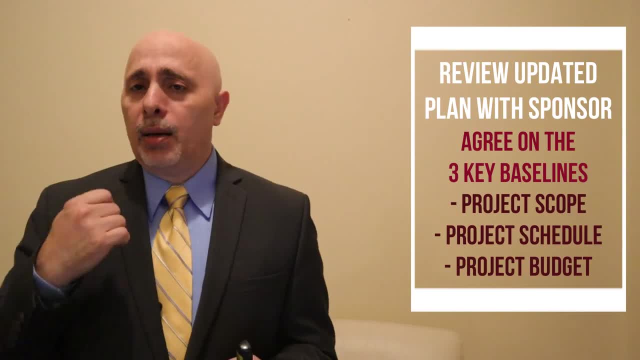 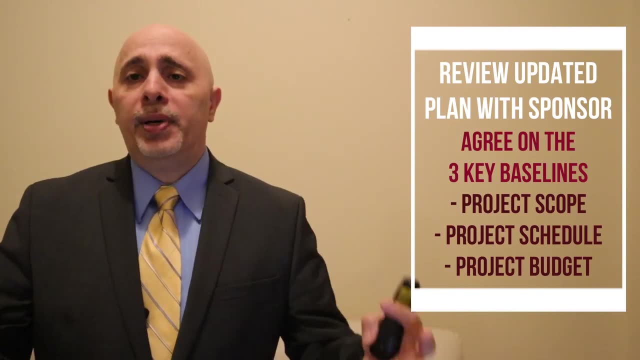 final schedule and talk to them about the budget requirements, how much they need to fund you on a periodic basis. what were the risks that you've identified, what actions you've taken to mitigate them. who participated in this risk mitigation process and then the final project plan And it 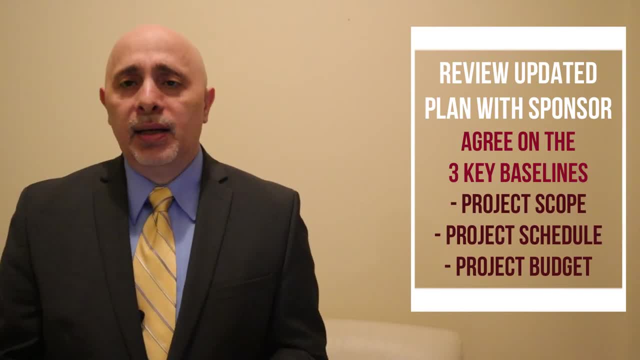 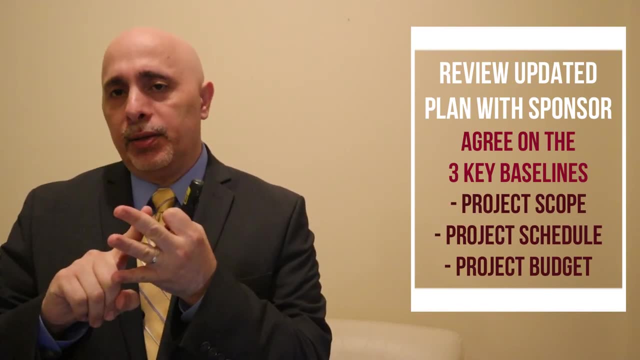 includes all of your project baselines. A baseline is an agreed to part of the plan And we usually talk about the scope baseline, the schedule baseline and the cost baseline. right Within the scope baseline, you could also include quality baseline, right. These are the ones that you want. 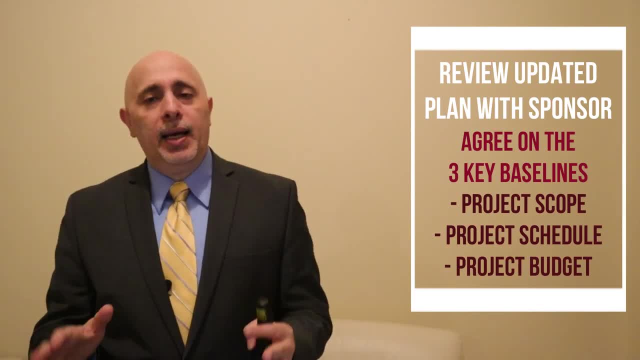 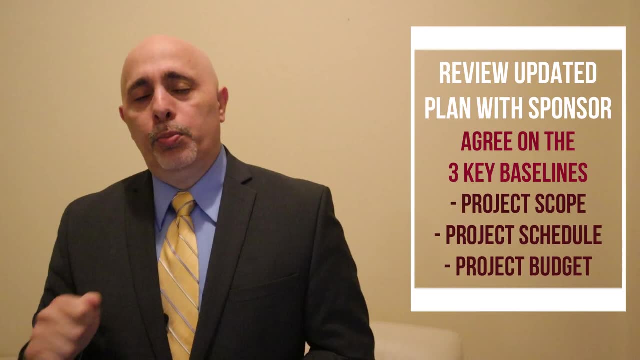 to agree to with your boss. Your boss looks at your plan, says: everything is good, I love what you did. And you say: all right, can you just sign off on this? Once they sign off, then your baselines have been signed up, And that was step number 14.. All right, so now what you have is a. 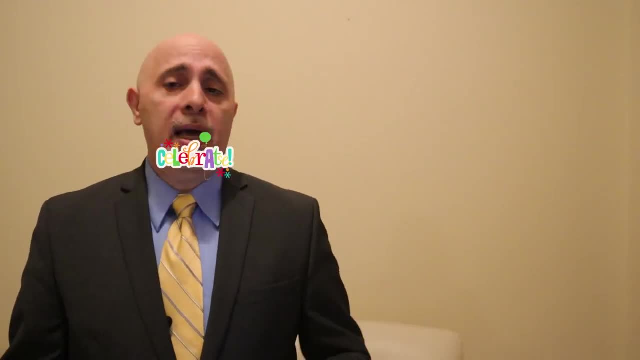 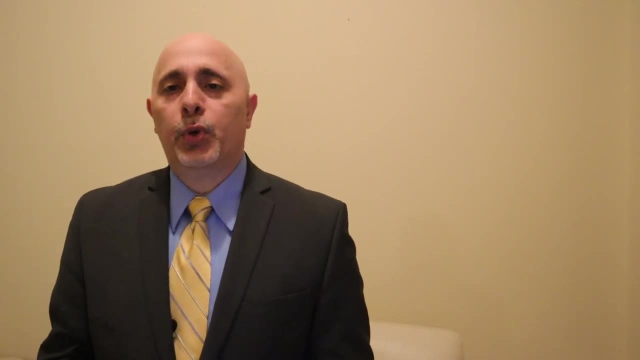 fully developed plan and your boss has agreed to it. The next step after this will be to go to execution, but that's for a different video. So I hope you enjoyed these 14 steps that I gave you in planning out your project. If you want to know more, if you 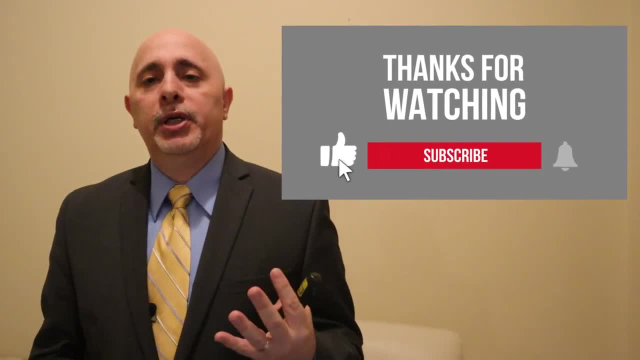 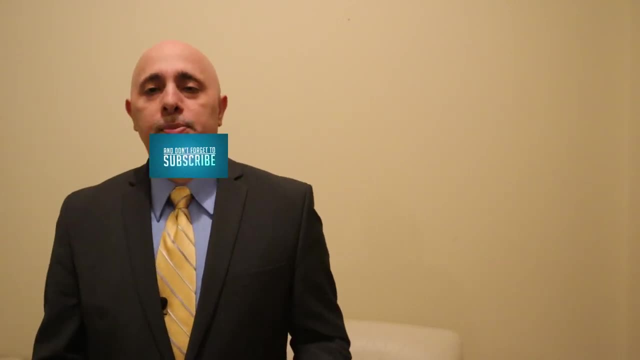 have any specific concern, talk to me. I am an expert in project management. I'll be happy to respond to you. Put your comments down below. If you like this video, please subscribe, And if you know others who can benefit from this video, please share While you're subscribing, please. 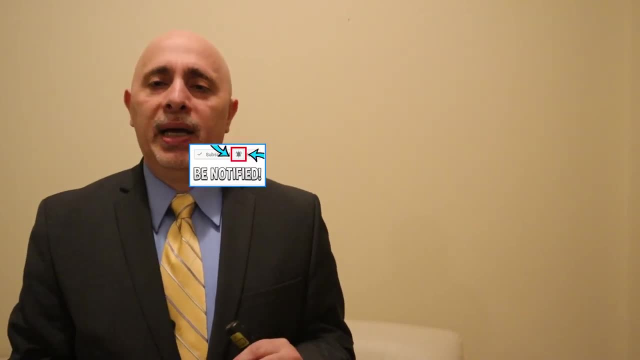 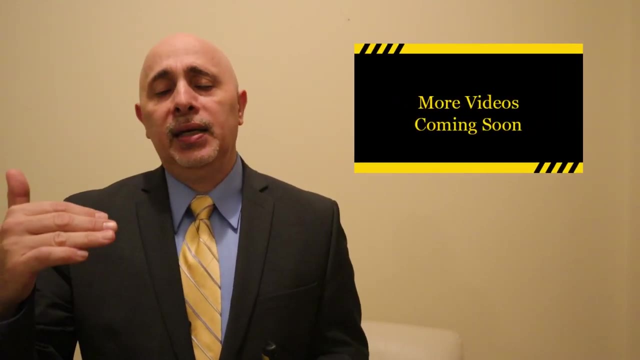 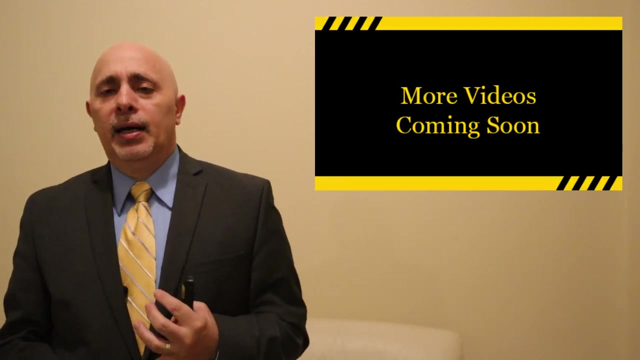 like this video, Make sure you hit the notification bell so you can be notified about new videos that will be released. I'll be releasing additional videos on all of the additional details about the 14 steps: the charter, identifying stakeholders, collecting requirements. There's already one.